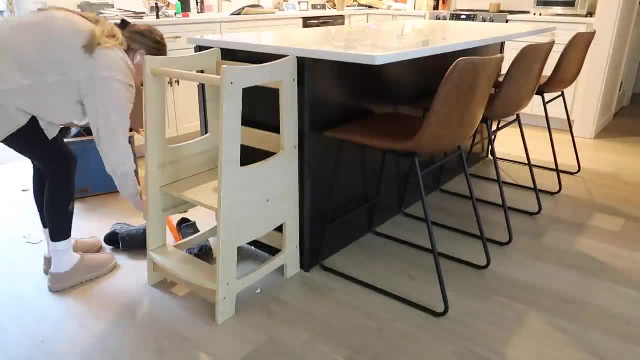 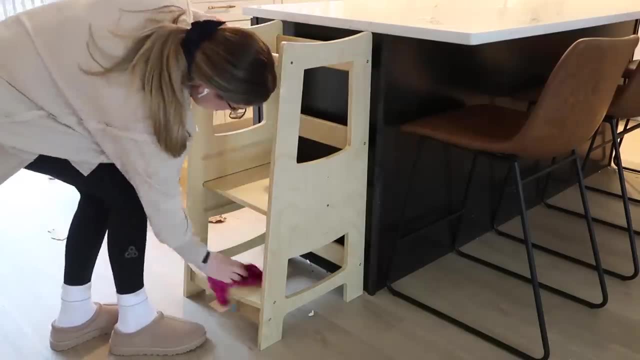 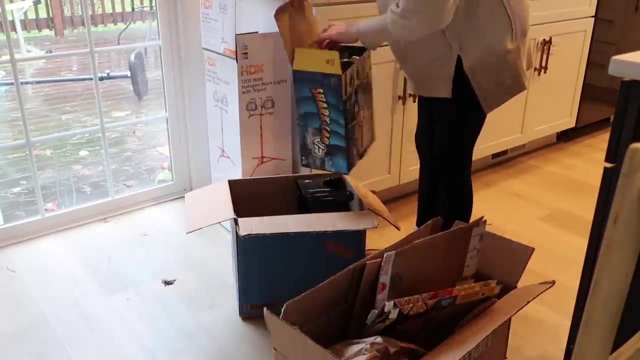 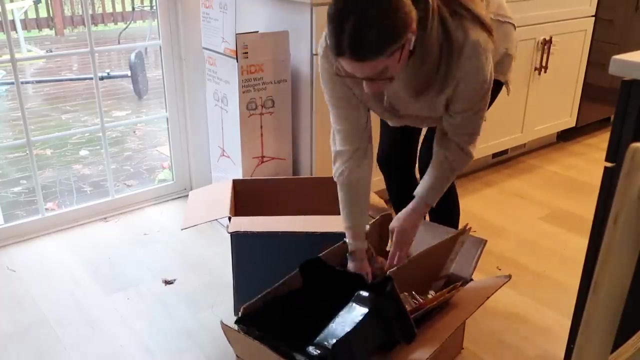 worth. it were the knockoff magic erasers that I got, but I believe I can get those, probably on Amazon. I've also heard some sketchy stuff about their company, so we are steering clear of Timu this year and forever. I filmed this video. 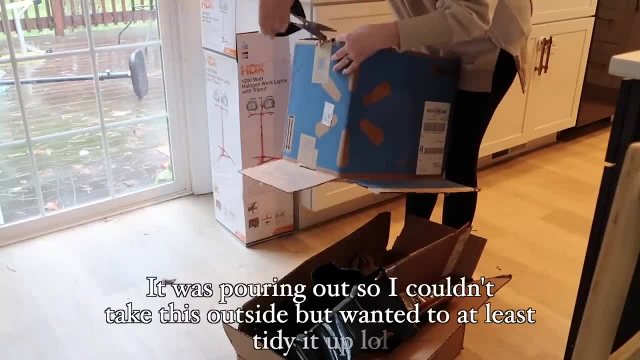 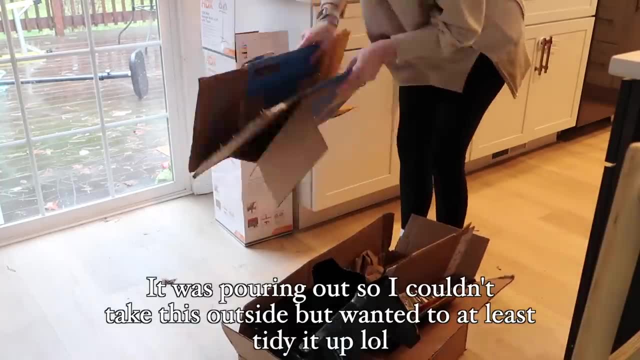 a couple of days after Christmas. so if you're wondering why there's so many boxes, that's why We just had a bunch of extra boxes laying around from opening up gifts. but that Home Depot box in the background is like work lights that we bought and we got those for the 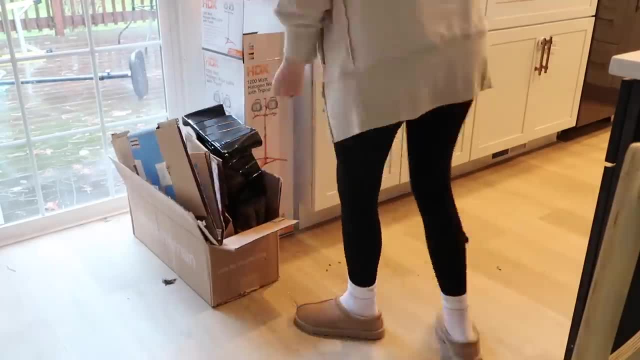 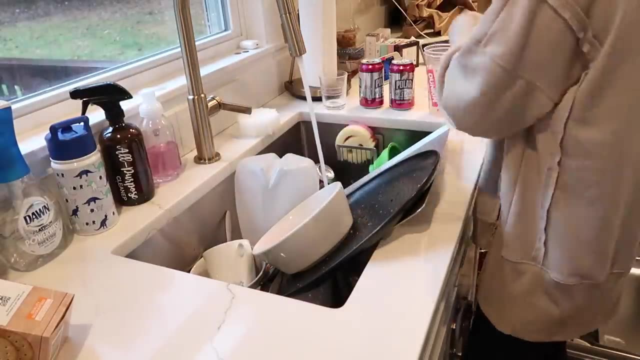 basement to help illuminate it, because pretty soon we are filming a huge, huge, massive, crazy basement declutter. It's gonna be a lot. so if you guys are looking forward to that, make sure that you subscribe to my channel and turn your notification bell on so you don't miss out on any of my new videos. 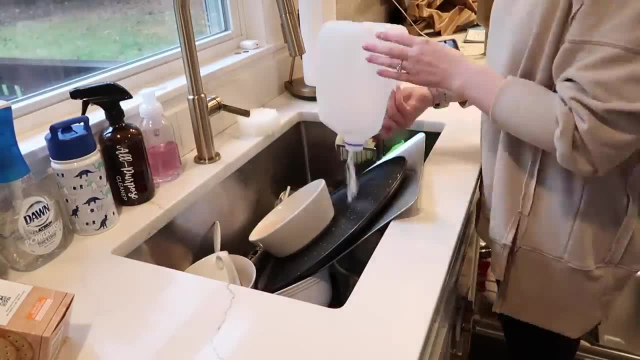 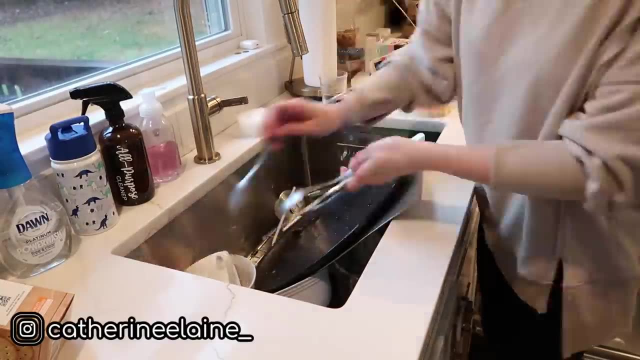 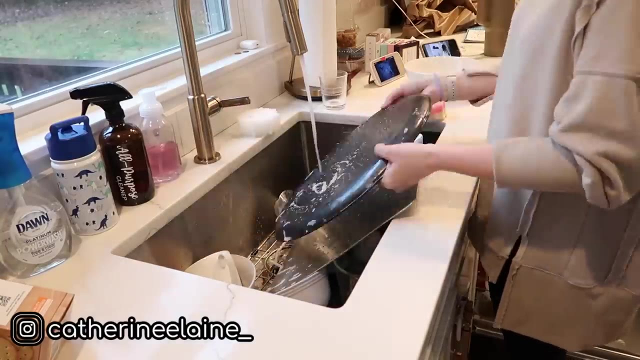 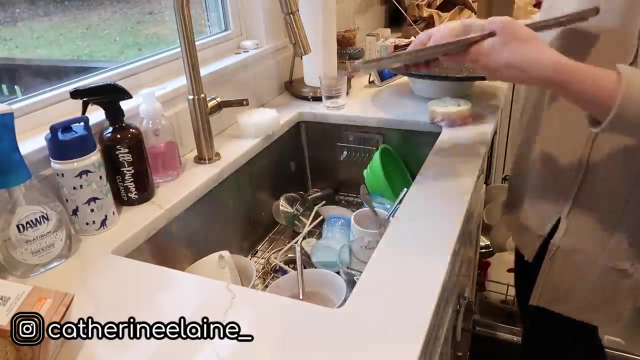 I'll see you guys in the next video. Bye. Another thing that I won't be buying this year is subscription streaming services. This is not physical clutter by any means, but it is so expensive, Even if you're only paying $5-10 a month. 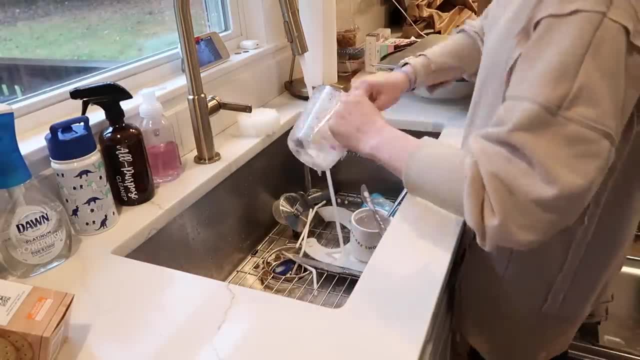 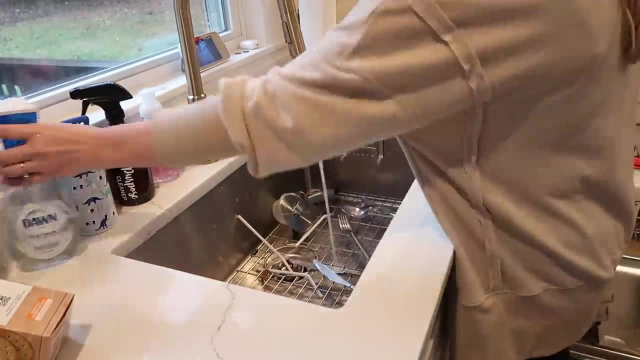 that adds up so quickly And we really don't watch a lot of TV in our house. We use YouTube TV for our live streaming and we have a Disney Plus and Hulu bundle and we don't need anything else. I think it's wild how we all 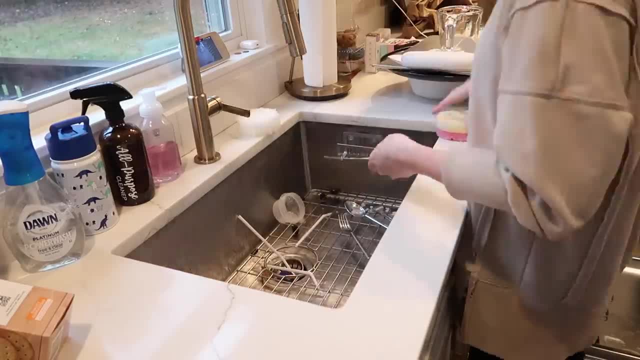 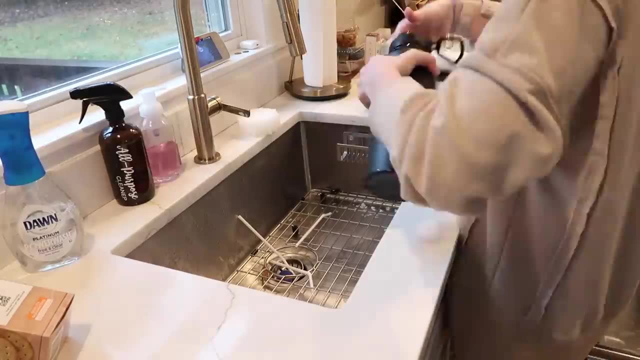 cut cable out to save money and then it totally backfired when networks split up into all separate streaming services. You guys will have to let me know what you use for streaming and if you have any tips or tricks to save money but still access the shows or movies that you want to watch. 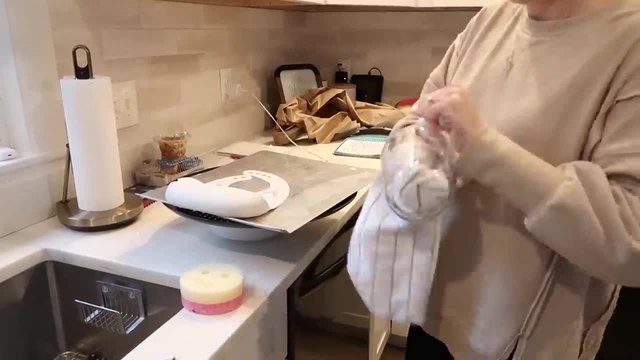 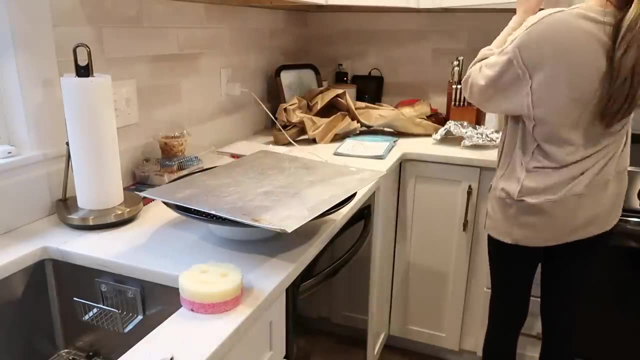 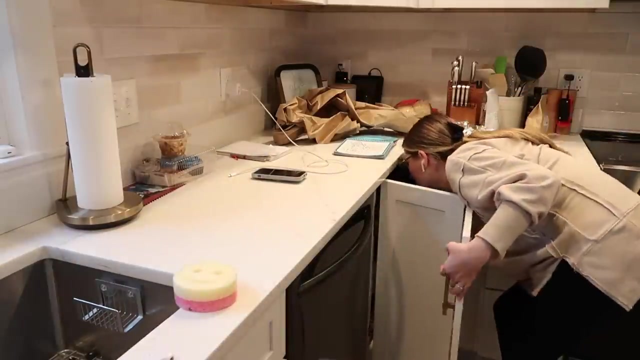 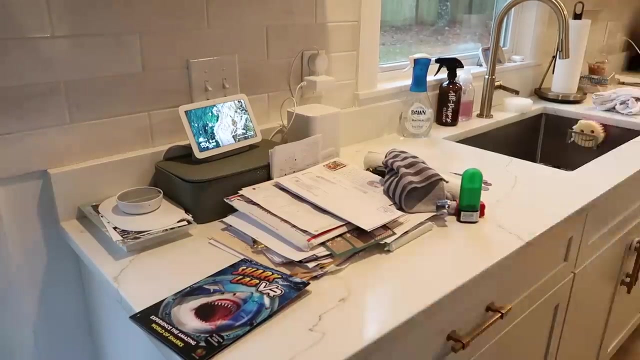 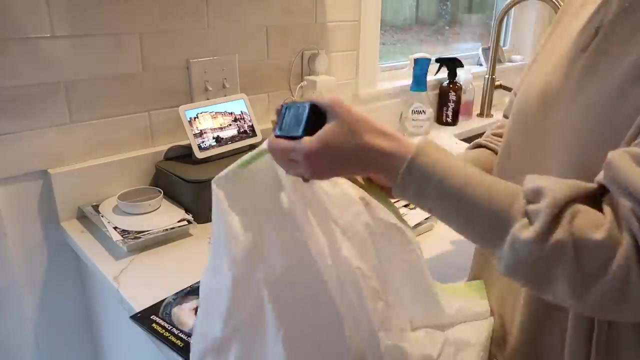 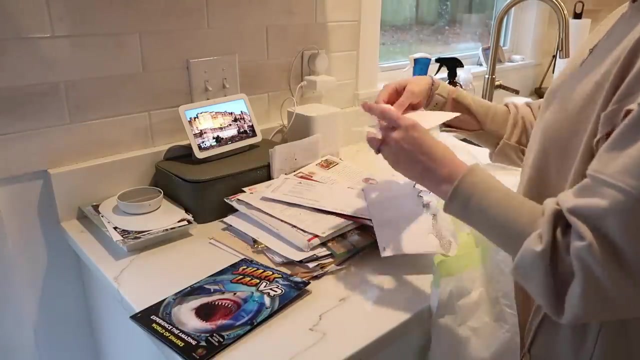 So the first area that we're going to declutter is this kind of clutter corner- is what I like to call it- in our kitchen. We just tend to throw a lot of random paperwork there and things like that, so I wanted to take out my trash bag and just start throwing things away that we don't need. 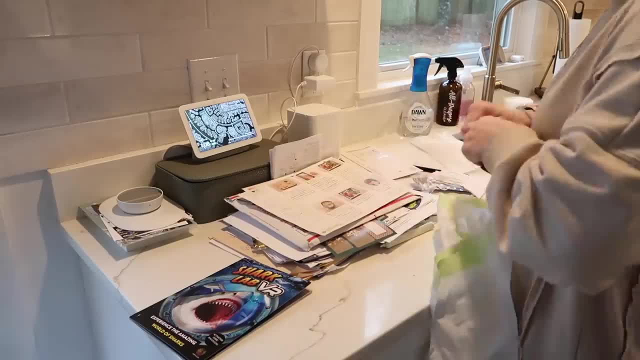 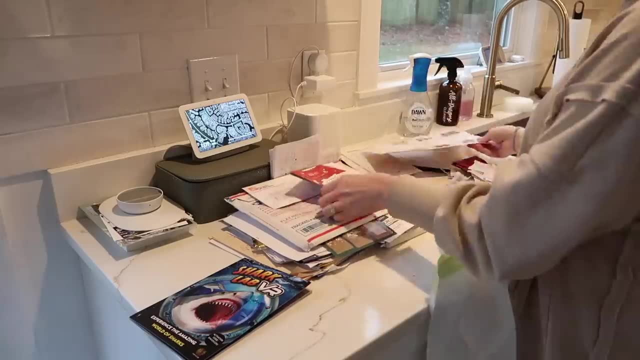 I was also creating piles out of this mess. so I was doing like an instructions pile, because there's instruction booklets that go to certain things that we have that I think we should probably keep, So I was putting those into a pile. I was doing a pile for things that needed to go into my little 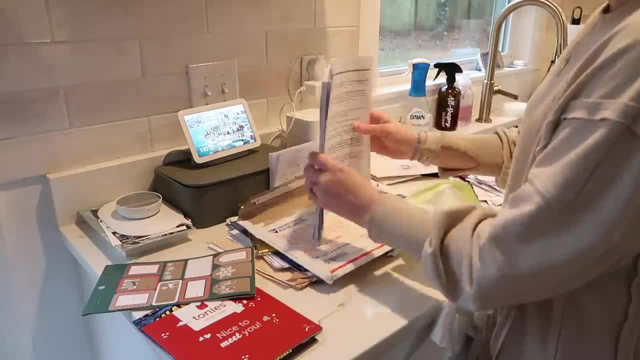 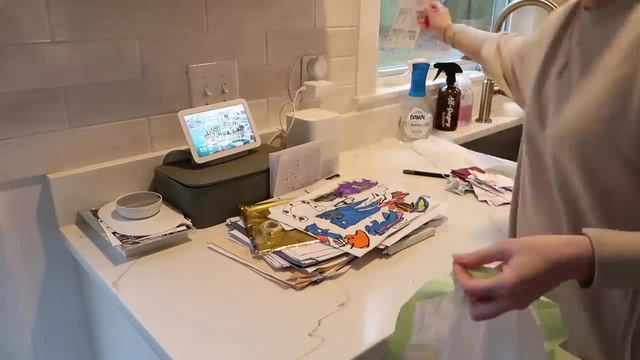 filing cabinet that I have, I was doing a pile of things that needed to go into the basement. So, yeah, some of this stuff is not necessarily clutter, because it's things that we do actually need. So I didn't throw away everything out of this pile, but I did get rid of a pretty large 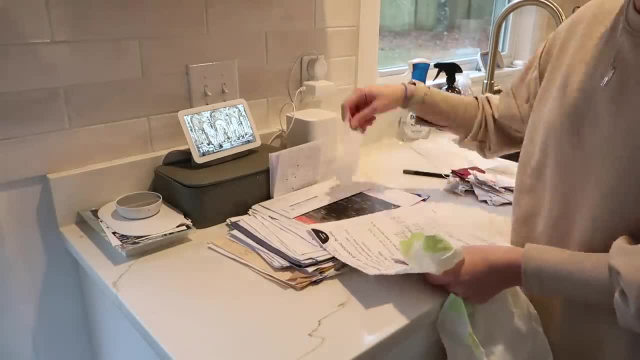 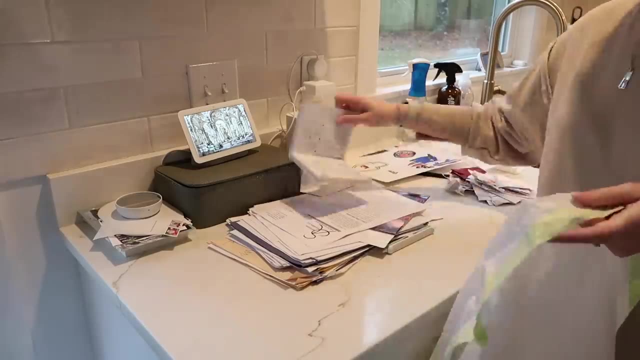 portion of it. I also wanted to go through the green bin that you can see here. So that bin is actually- I think it's called- a photo box, and I really like using those for my countertops in particular, because sometimes you have things that you want on your countertops or you just don't. 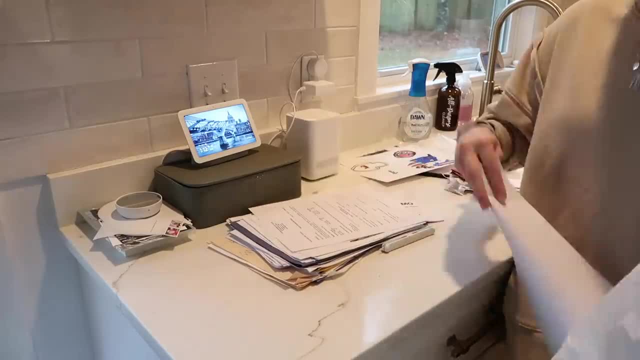 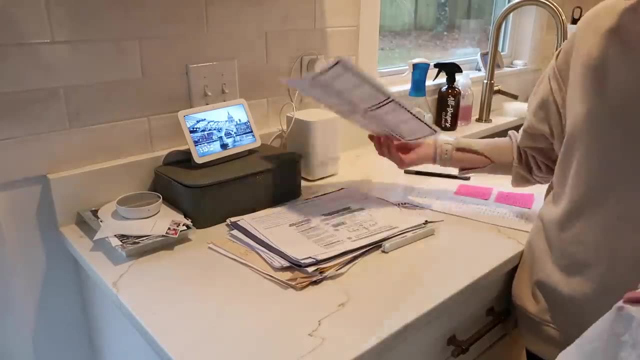 have a place for, but you also don't want it to look like clutter all the time, So I wanted to. so having a photo box is just an easy way to kind of consolidate those miscellaneous items so they don't look so bad on your counter, but they're still there if you need them. 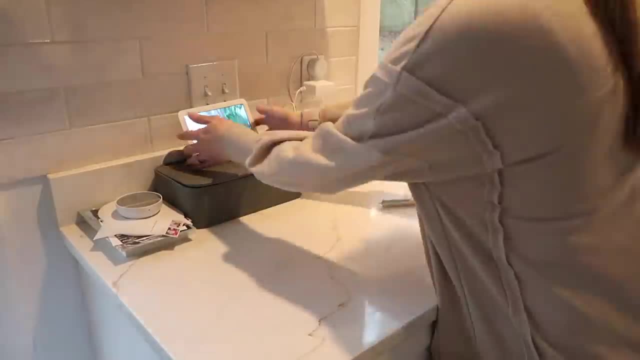 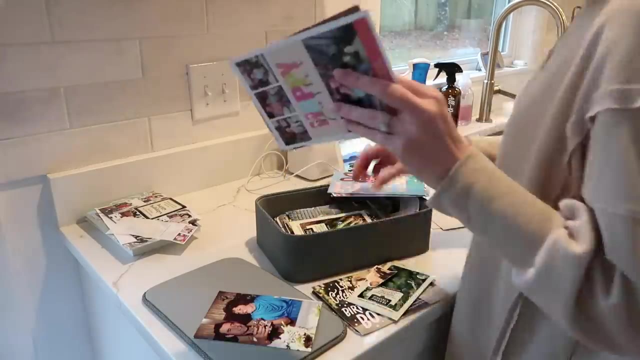 In this case, however, I do actually store photos in this photo box, and do I need those on my kitchen counter all the time? No, but I honestly don't know where else to put them. so I would love to know in the comments what you guys do with, like your Christmas cards that you receive from family. 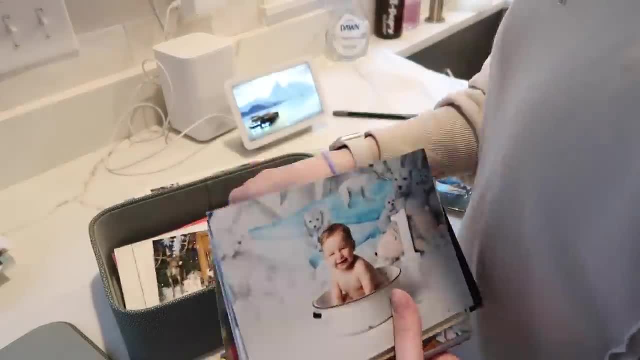 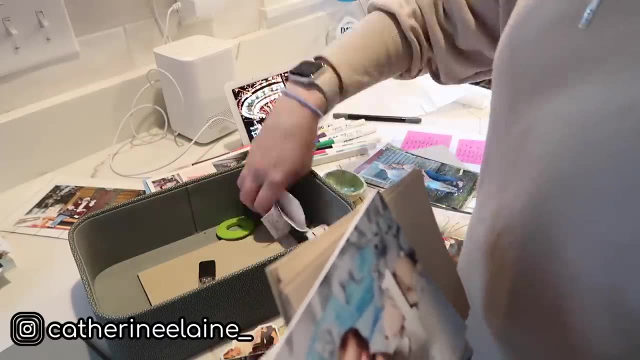 and random photos that you have and stuff like that, because this is what I've been doing with it and I do actually like having it there so I can look through them if I want to, but I just don't know if this is like the long-term solution. 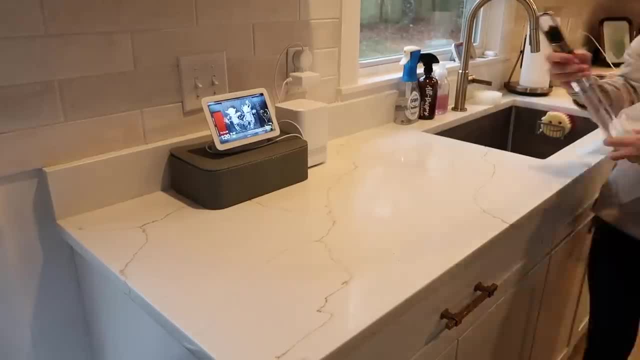 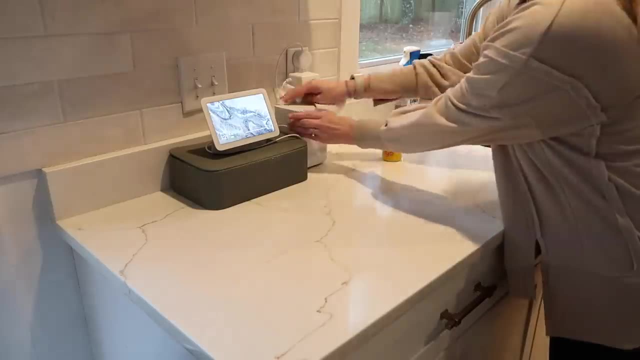 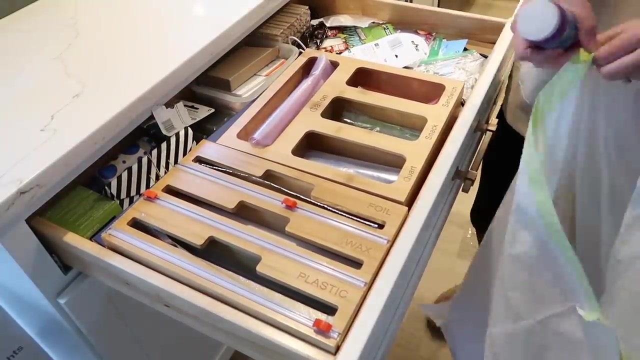 Now that we have thrown a bunch of stuff away and then put a bunch of things back where they actually belong, we are going to start opening up drawers in my kitchen so I can declutter inside of those. This drawer is where we obviously keep like tinfoil and ziploc bags and things like that. but 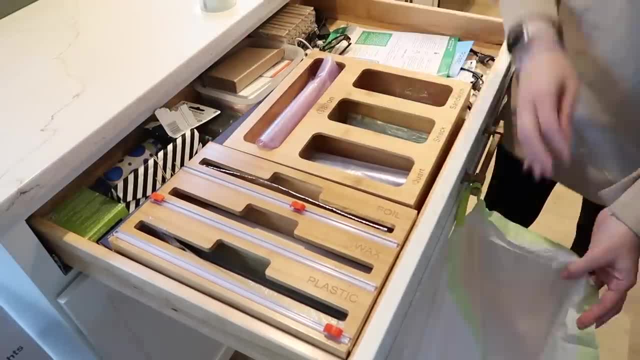 for some reason, it also always collects junk. so I'm going through all of the junk that's in here. I think I'm going to put a lot of stuff in here. I'm going to put a lot of stuff in here. I'm going 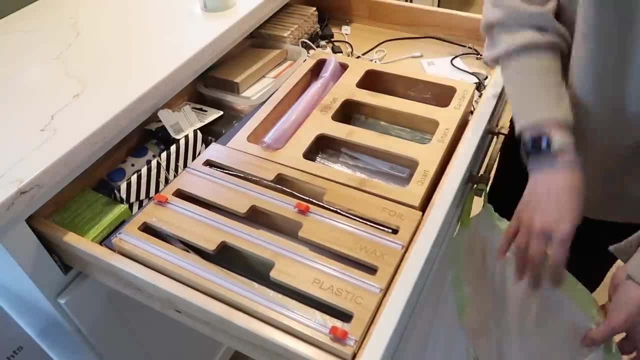 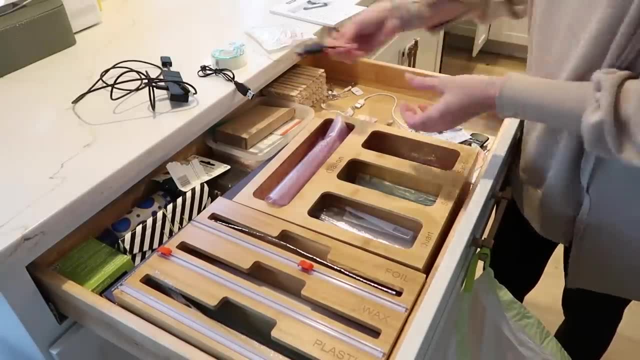 to throw away a good portion of what was in here, and then we can actually store our cutting boards in here, which is what we usually do, but there was just no room for them anymore, so this felt really good to go through. Also, I have a million cords that I don't know what they go to, and I'm so. 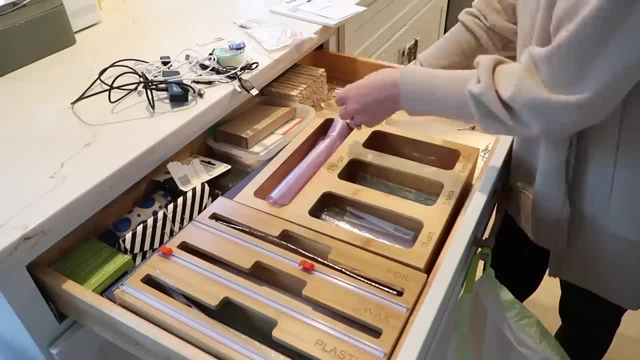 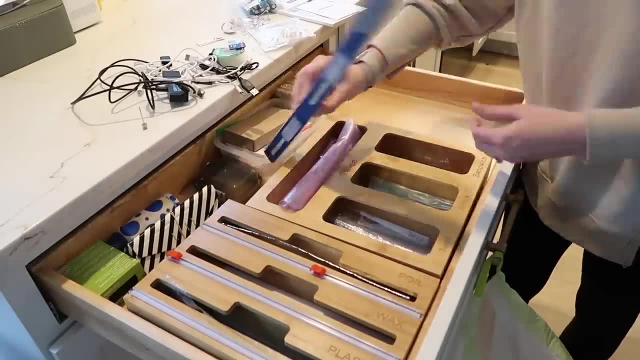 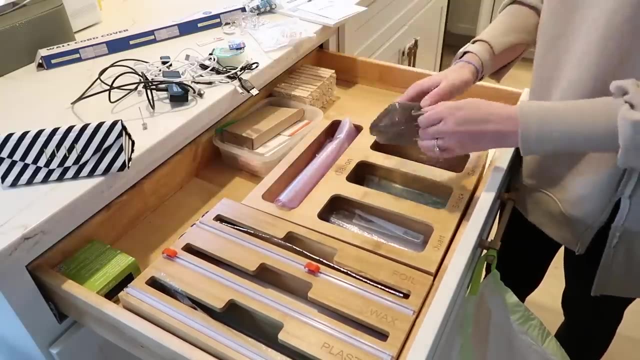 afraid to throw them out, because what if I need one? So I'm curious: do you guys also have cords all over your house and what do you do with them? Something else that I don't plan to buy in 2024 is home decor. I feel like social media has really 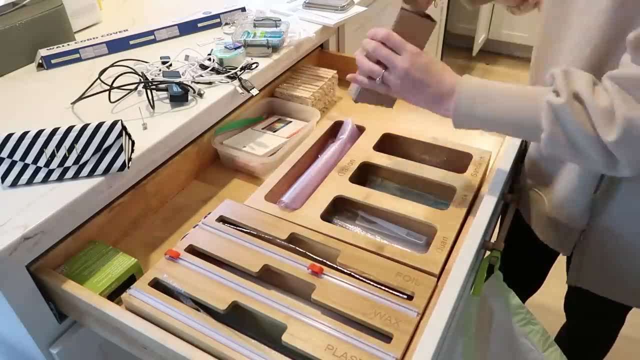 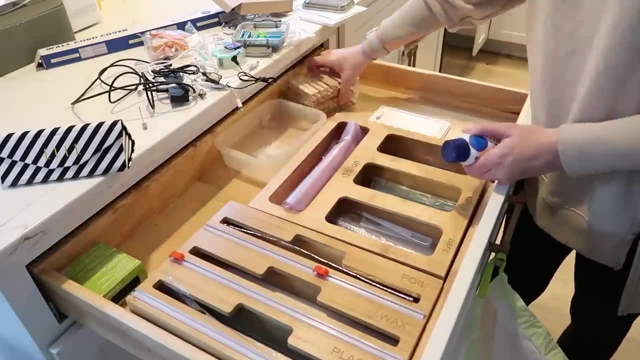 caused us to feel like our homes aren't enough and, if we don't go all out for every season, that we're somehow lacking or missing out. I find myself comparing my home and my things all the time to things that I see on social media, but what you see online is such a small percentage of what real 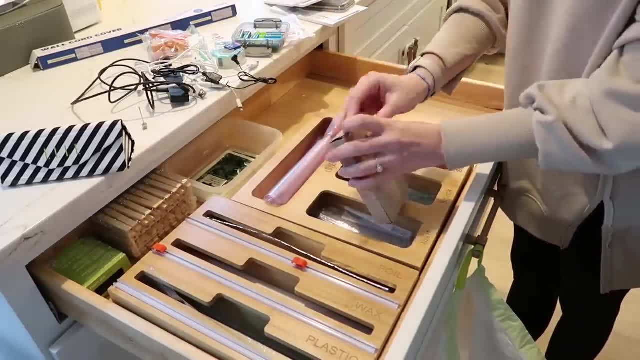 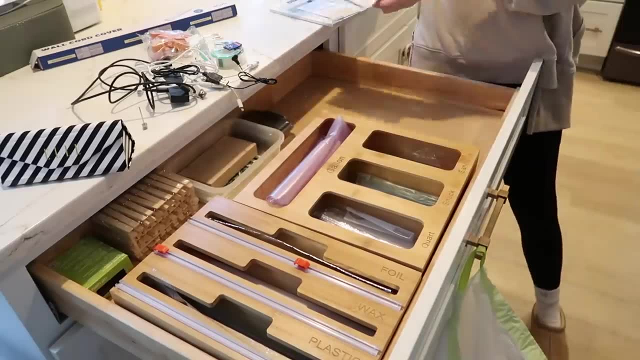 homes actually look like. Sometimes I feel like, because of my job here on YouTube, I have this requirement to buy a lot of things that I don't want to buy. I don't want to buy a lot of things to keep up with the trends, to stay interesting, but I don't want to be that way anymore. I'm just a. 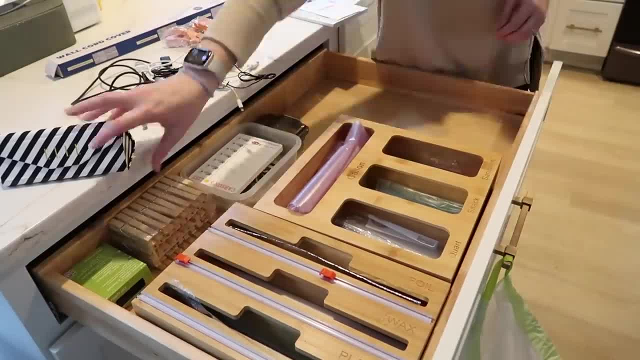 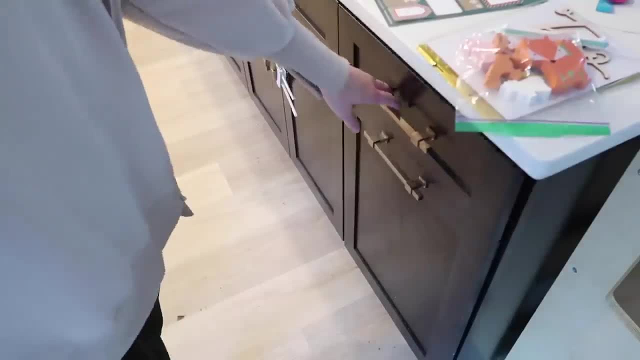 regular mom living my regular life. We are doing some traveling actually this year, in 2024, and I'd so much rather just put my money towards my family's memories than to spend it on useless home decor that will just collect dust and create more clutter in my home. 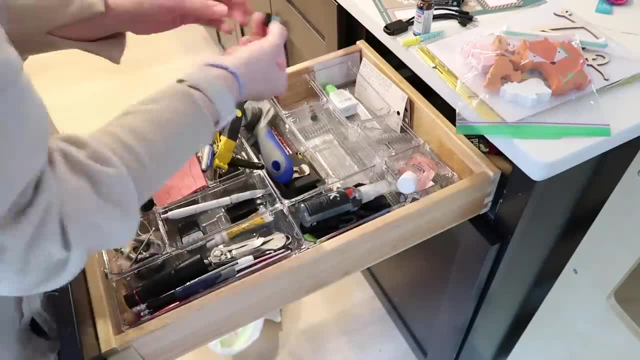 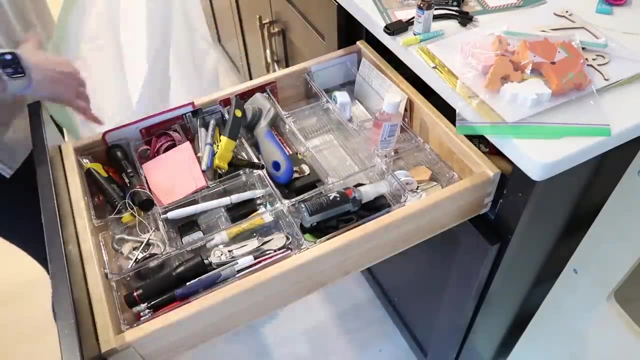 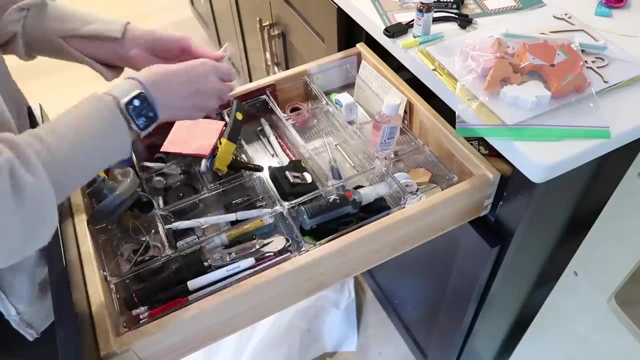 This drawer. who knew it would create such a stir? This is our junk drawer or utility drawer, whatever you want to call it, and I've mentioned this in past videos. but sometimes when I organize this drawer in a video, I get comments saying that my home is not organized because anyone that has 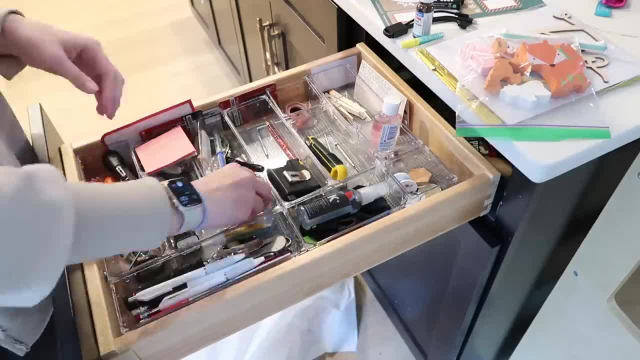 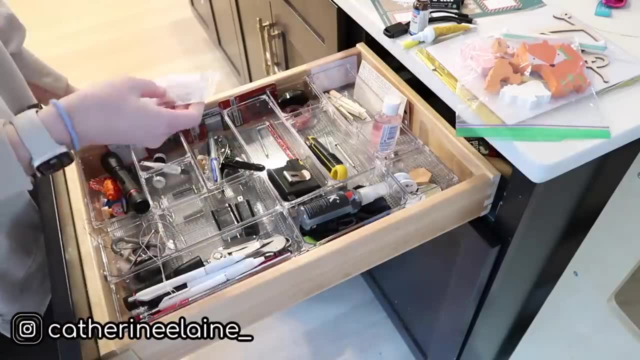 an organized home should not have a junk drawer. I don't know what these people have against junk drawers, but I'm a big fan of them. If you live in a home like mine, where you don't have a dedicated office room, you don't have a lot of space. you don't have a lot of space. you don't have a lot of. 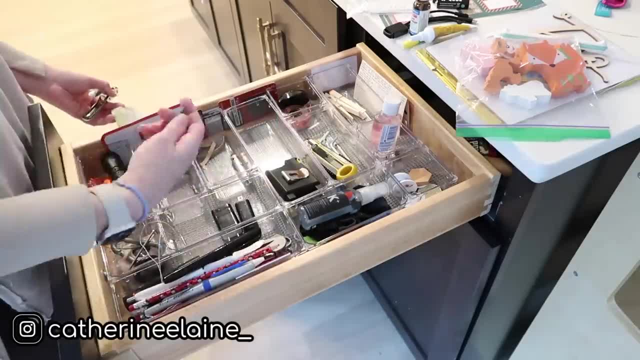 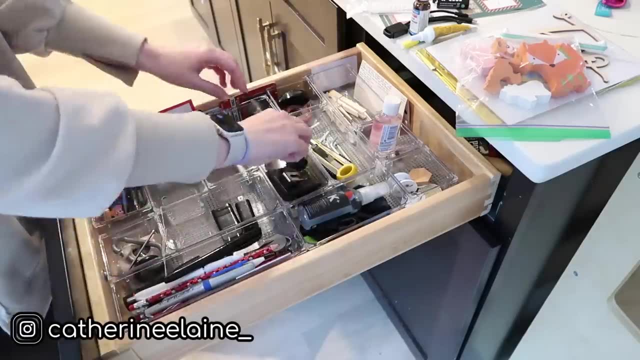 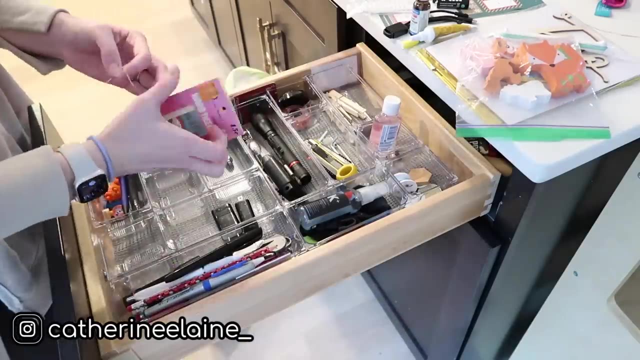 room, or you don't have a garage. then there are just certain items that you don't have a proper home for, and I want these things to be accessible to me. I reach for them all the time, so it's to me it just makes perfect sense to have a junk drawer in our kitchen. Ours was getting very cluttered. 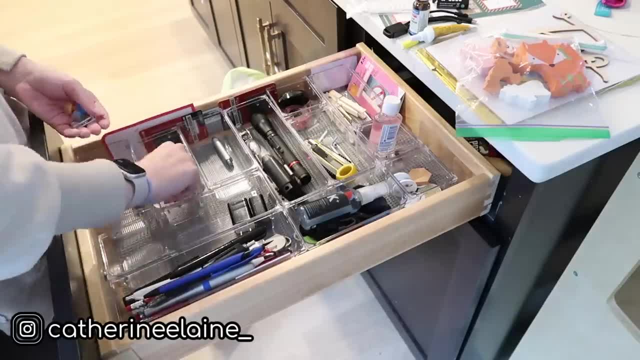 My six-year-old goes in here a lot, my husband goes in here a lot, and they don't necessarily put things back into the space where they belong. so I needed to get everything back into its proper spot and then just put it in the right place. I don't want to have a junk drawer in my home. 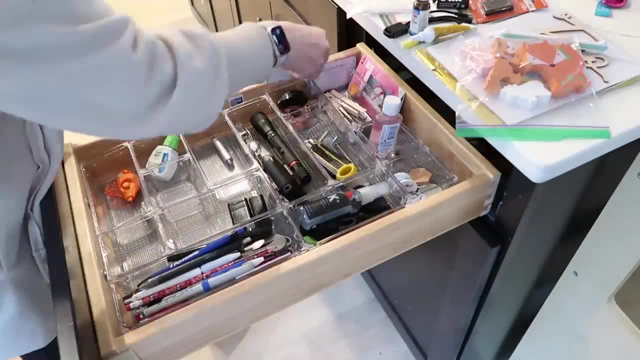 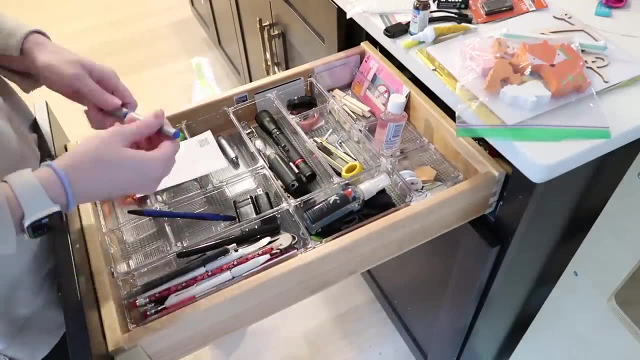 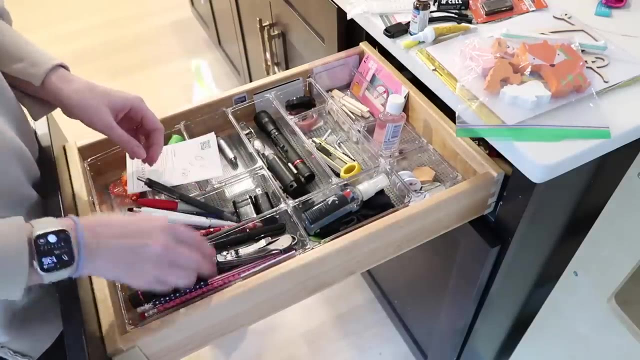 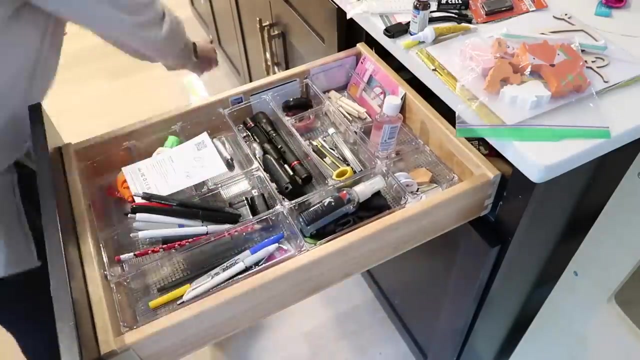 Just get rid of all the trash and random junk that had accumulated over time. I feel like there's this common misconception that once you've organized a space or decluttered a space, that it should remain that way. but that's just not realistic. We do the best we can, but 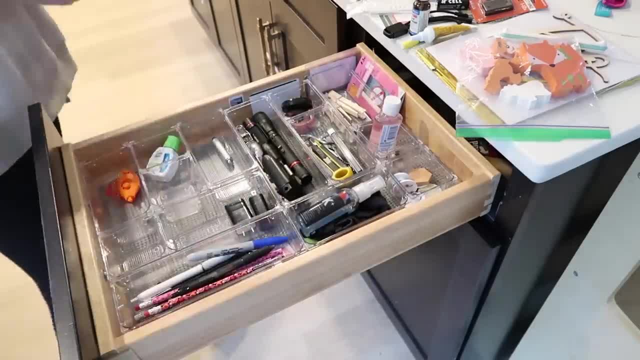 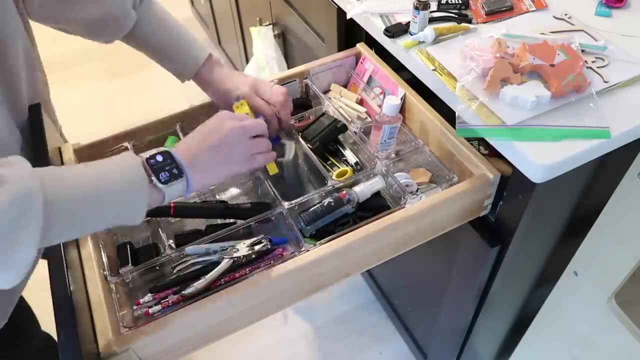 we're just again normal people Over here living normal lives, and moral of this whole story here is that you're going to have to revisit a space, probably multiple times and over and over again, even if you think you've come up with the organization system. that's going to last. 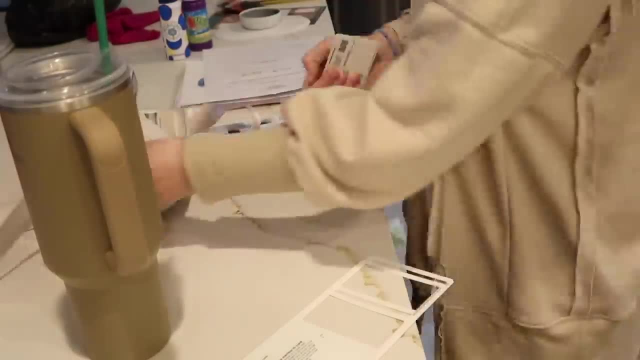 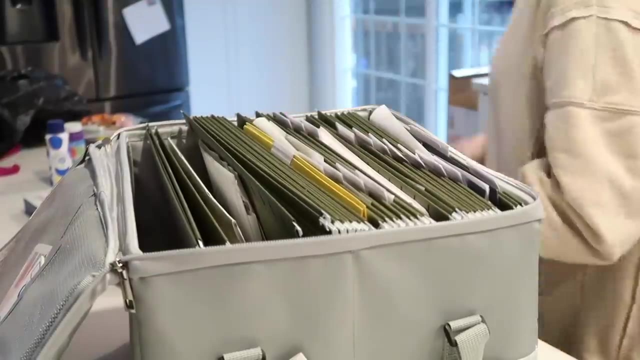 We had some new insurance cards that I had sitting around. I was afraid they were going to get lost in the shuffle, so I wanted to get those put away into my wallet for when I need them, and then I'm just organizing all the rest of the things into our little filing cabinet that I had. 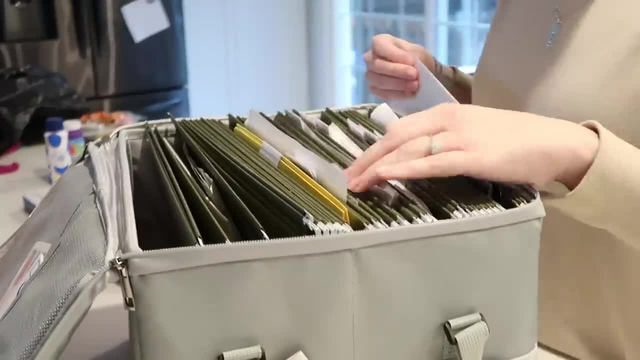 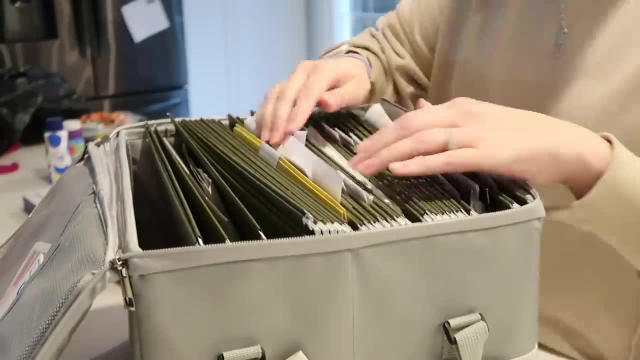 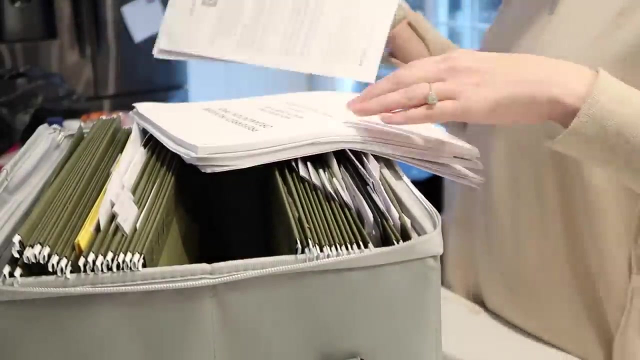 taken from that pile on the other counter. earlier I got this little filing system off of Amazon, I think, and I will try to remember to link it down below, but we really like this and it's helped a lot with keeping track of our papers. We still do collect so much paper clutter because we have a 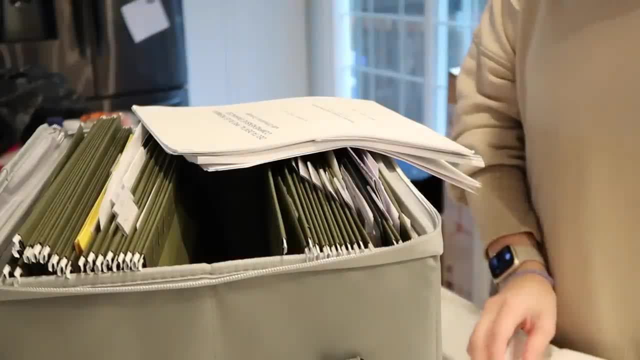 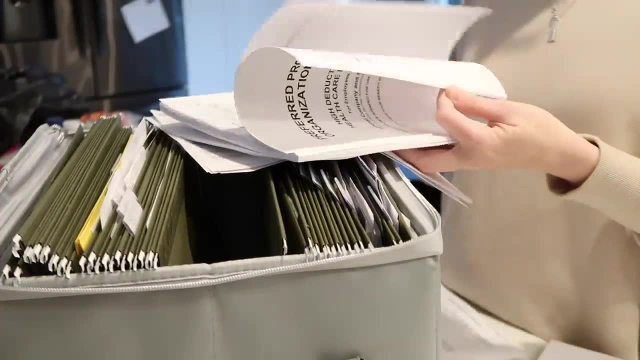 school-aged child who just brings home so much schoolwork. but actually I do have a video planned where I'm finally going to take a look at it and I'm going to show you how to do that. So if you're not subscribed to my channel, make sure you do that so you don't miss all these videos I have coming up. 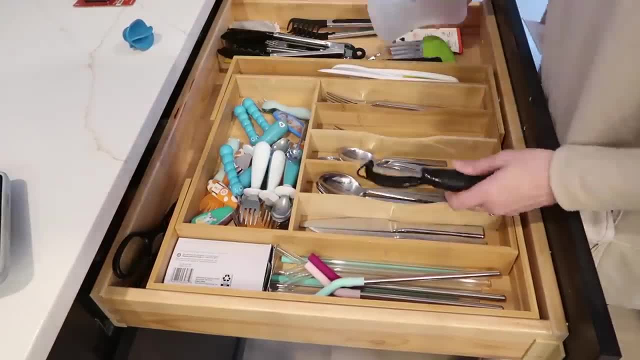 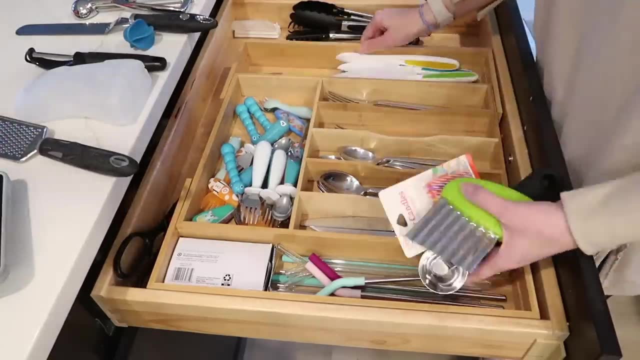 Moving on to our cutlery drawer here. I just took out a couple of things here to get rid of, and then we're going to open up another drawer right beside this one, and that one really wasn't too bad, Didn't need to do that. I just took out a couple of things here to get rid of and then we're going to open up. 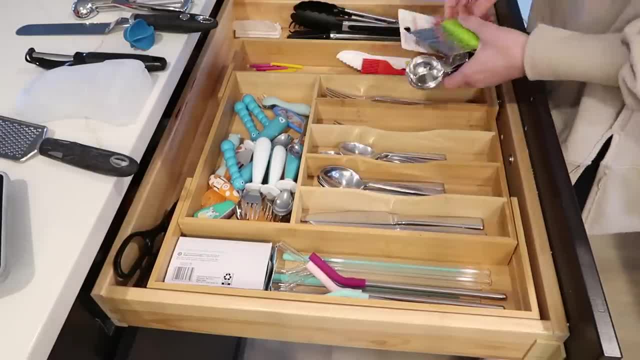 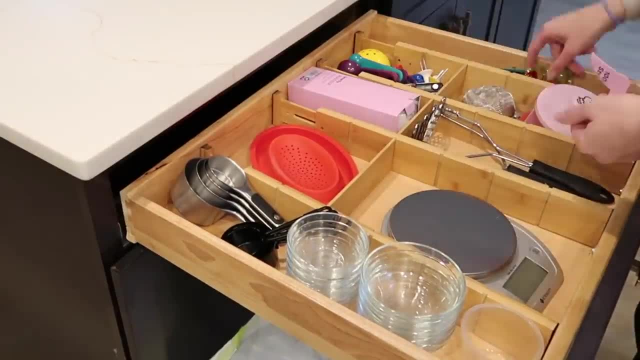 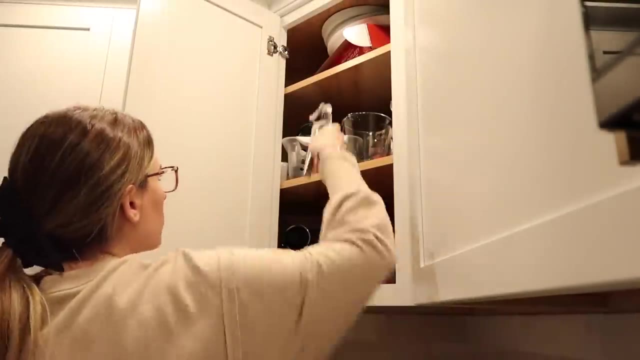 another drawer right beside this one, and that one really wasn't too bad. Didn't need to throw away too much stuff, but I did get rid of just a few things, and every little thing counts in reducing the clutter in our home. This corner cabinet here holds a bunch of our stainless steel cups and 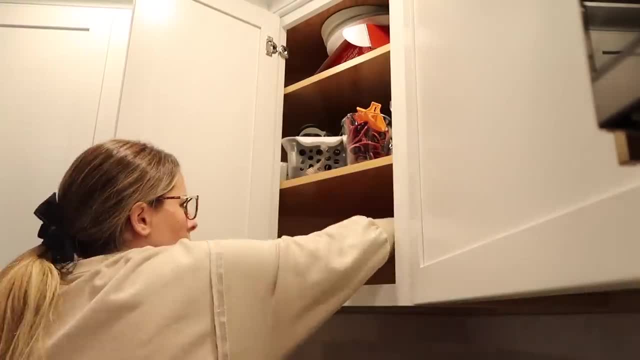 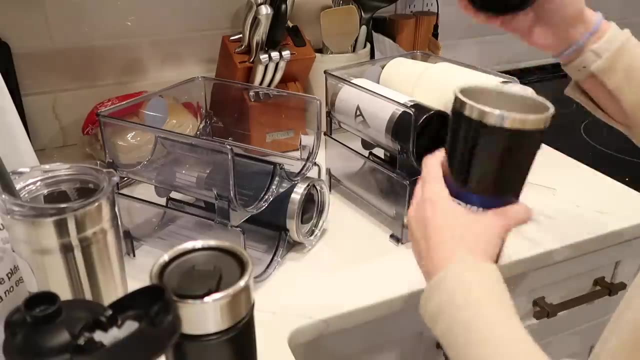 I've tried to declutter these a couple of times and I feel like we just always accumulate more of them. and it's not that we're buying them, We're being, like, gifted them and I don't know. they just continue to collect dust in our cabinet. So I'm going through them and again, I'm ruthlessly. 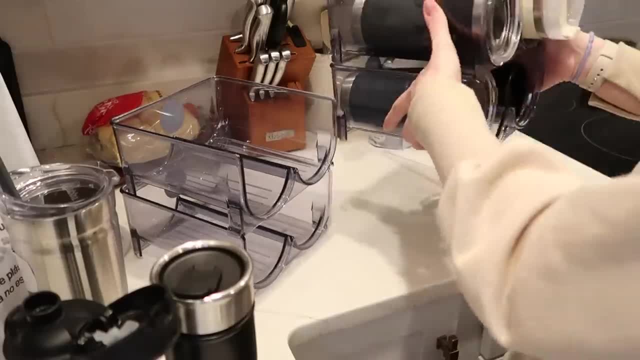 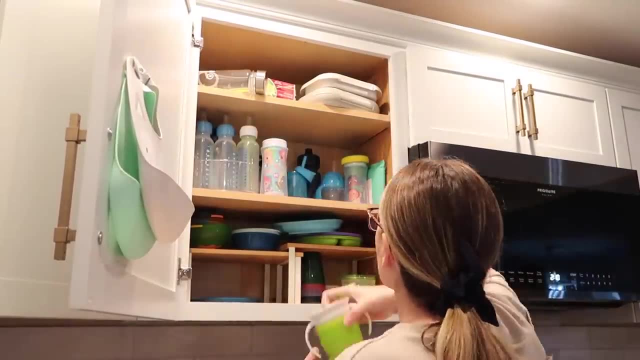 decluttering today, so I'm getting rid of a whole bunch of these. Some of them were missing parts or they were just super old and just had been worn down, so I did go ahead and get rid of all of those and it felt so good. and then we're going through the kids cups as well. We had a couple of cups in. 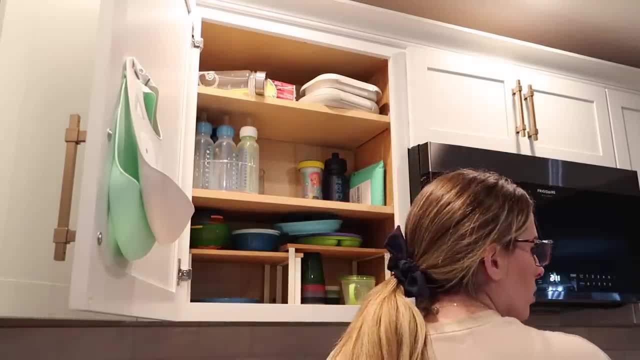 here that I just straight up hated because they leak everywhere. but then also, Sutton is no longer using bottles, so I was going to get rid of them, and then I'm going to get rid of all of those. So I'm going to get rid of all of those, and then I'm going to get rid of all of those. So I'm going to. 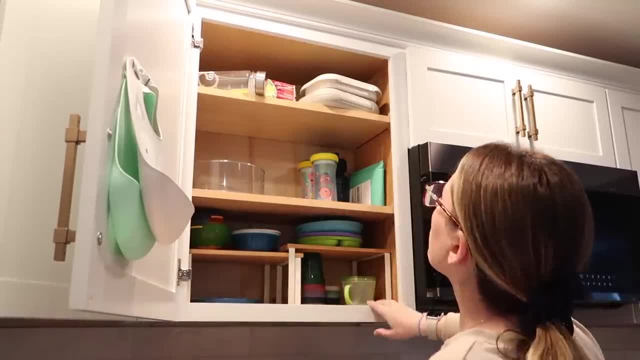 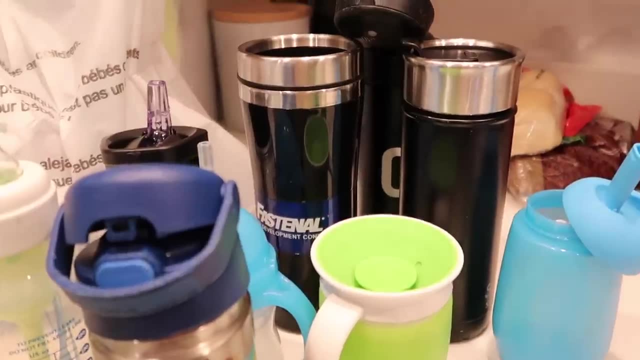 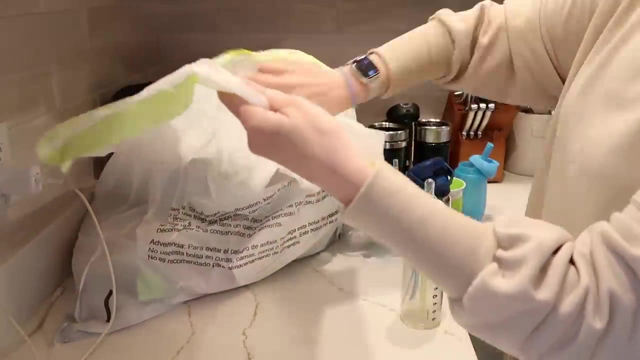 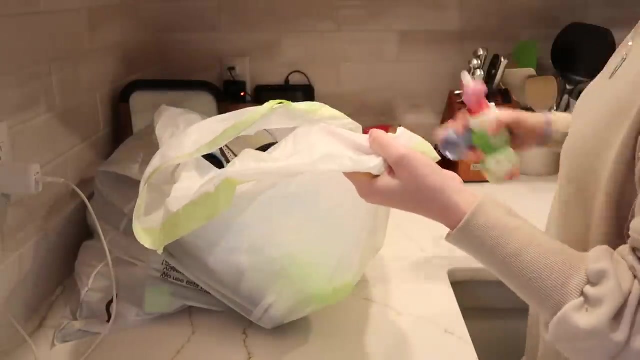 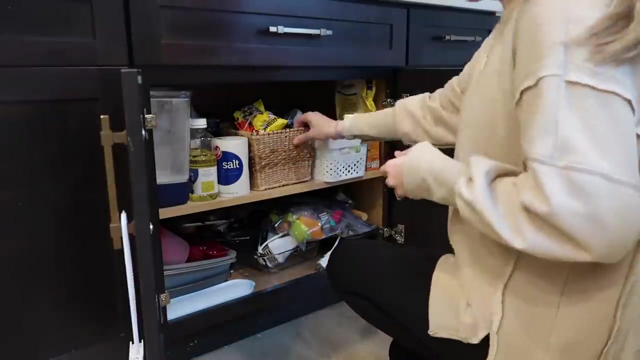 get rid of all of those, and then I'm going to get rid of all of those. So I'm going to get rid of all of those able to declutter all of those bottles. So I'm going to get rid of all of those bottles. 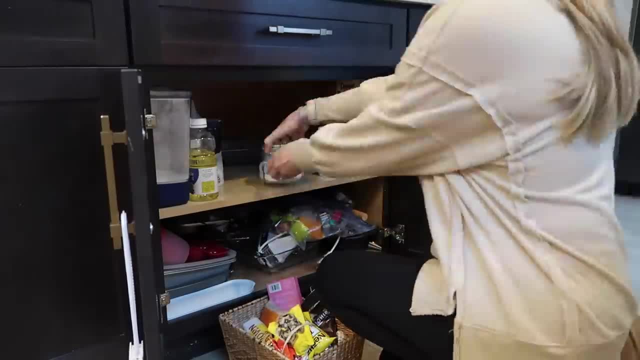 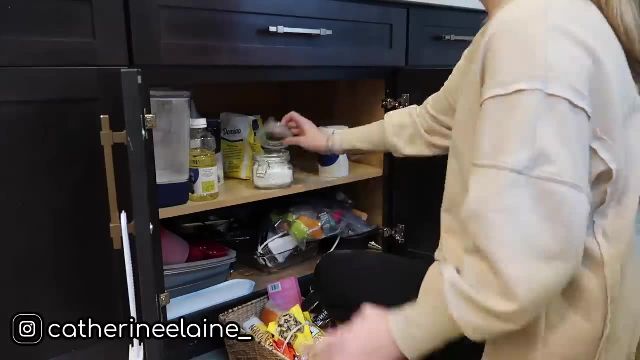 that I wanted to get rid of, but there really wasn't too much. I organized this. I want to say it was a few months back, but it may have been even longer than that and so far that system that I've been using- while it doesn't look the prettiest ever, it's been working pretty. 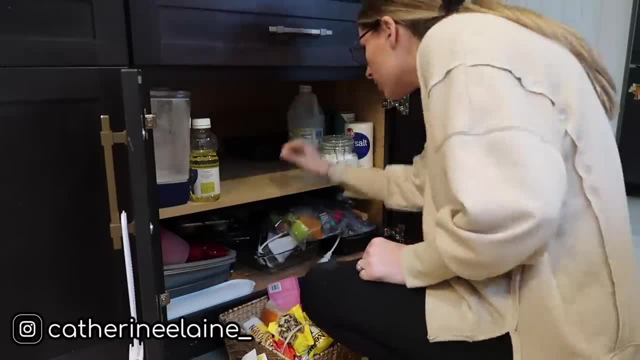 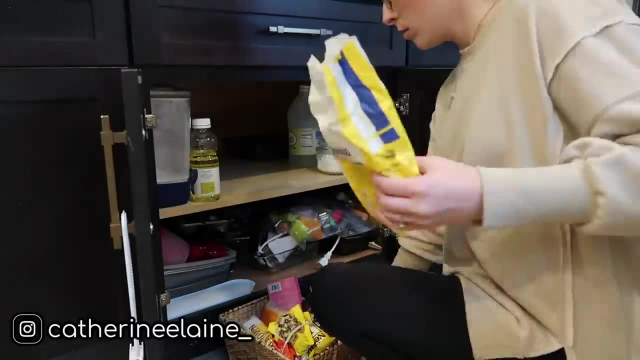 good. but over Christmas I did a ton of baking and things kind of got shuffled around. so I wanted to go through this cabinet and consolidate any ingredients that were just kind of loose laying around and also get rid of anything that we may no longer need. And since we're talking about things, 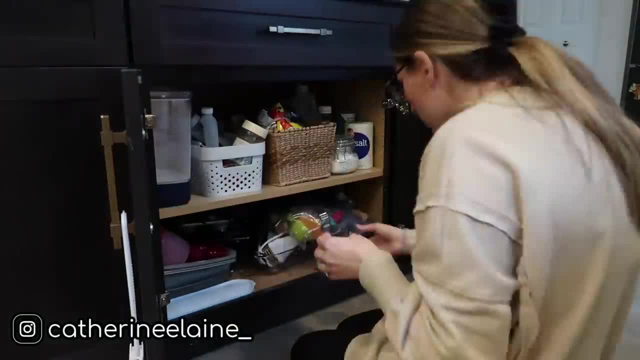 that I want to get rid of. I'm going to get rid of all of those. So I'm going to get rid of all of those I won't be buying in 2024.. One of those things is baking supplies, because I have more than I could. 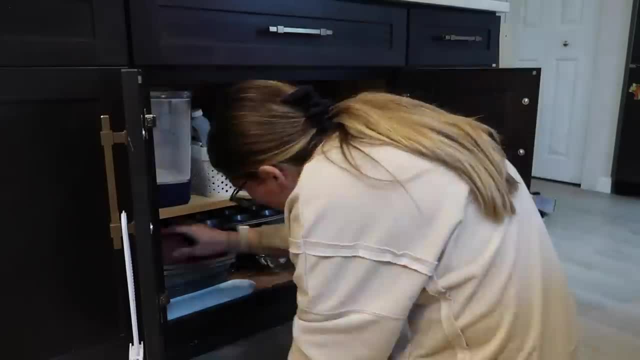 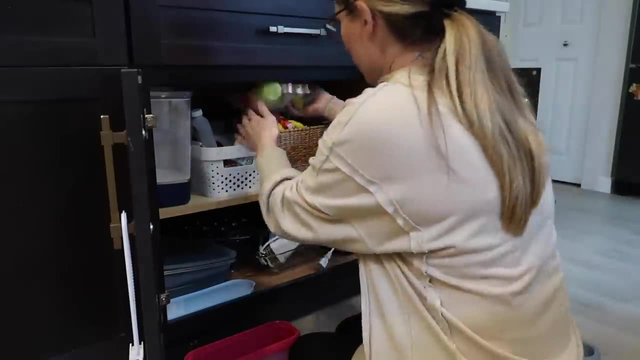 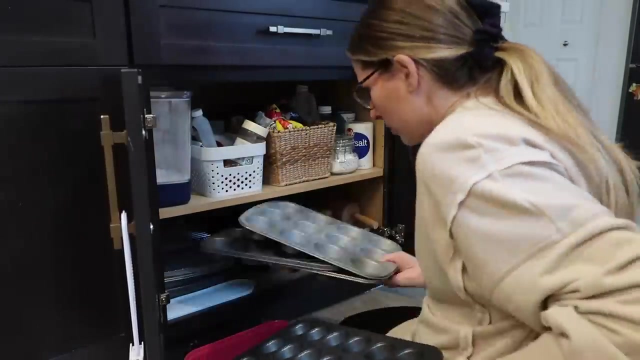 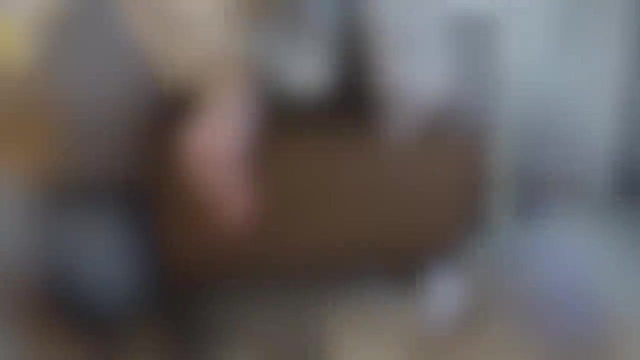 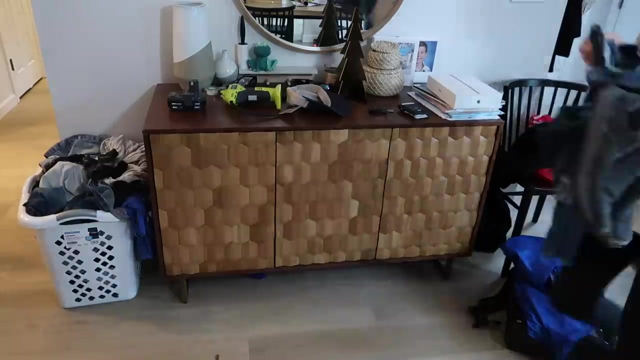 ever need, and I don't bake enough to justify buying anything else. This area of our home was driving me crazy. It needed to be picked up first of all. There was just stuff here that obviously didn't belong, but there was also a lot of clutter in here that we 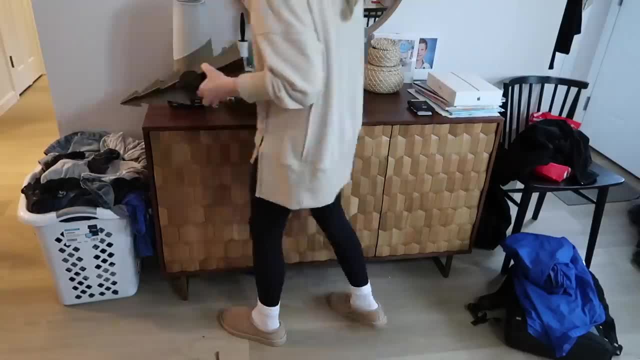 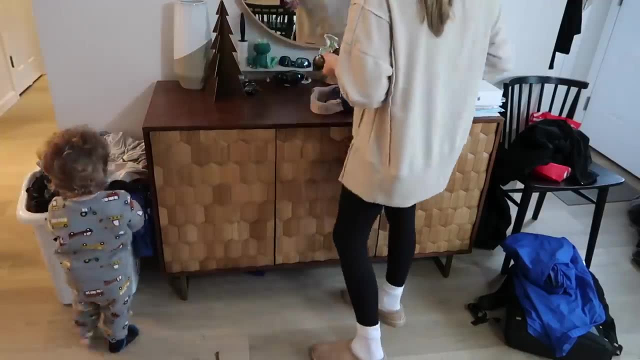 needed to get rid of. This is not trying to clean with a toddler, then I don't know what is, because everything I tried to put on this laundry basket for my husband to go put away, he just kept grabbing and I had to like keep moving it around. He's always into everything these days, but we're 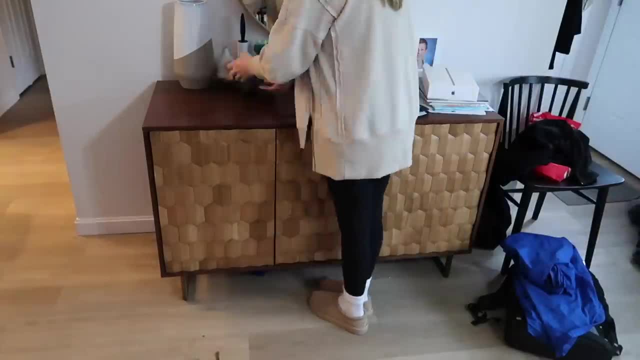 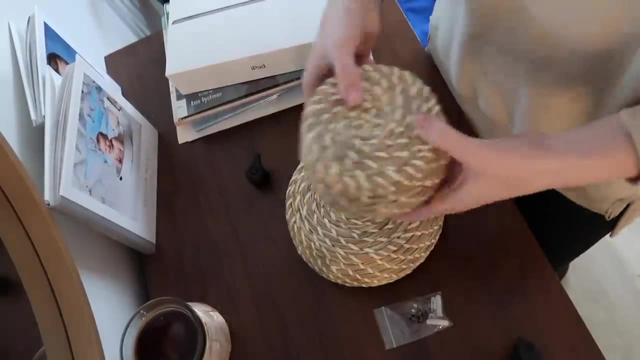 throwing away these sunglasses. I threw away a couple of my old sunglasses. I threw away a couple of my other things already. There was like a pair of shoes of my husband's that were totally worn out and needed to go. And now we're going through these bins that I got years ago from Ikea. I 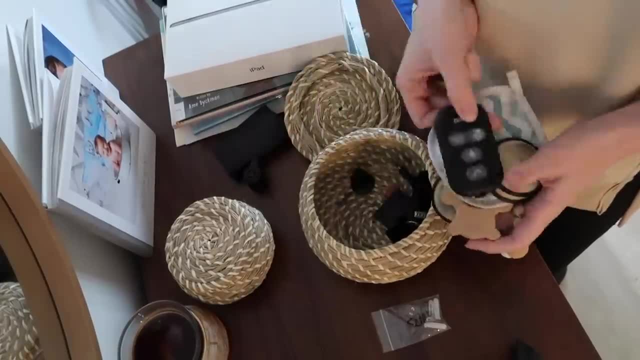 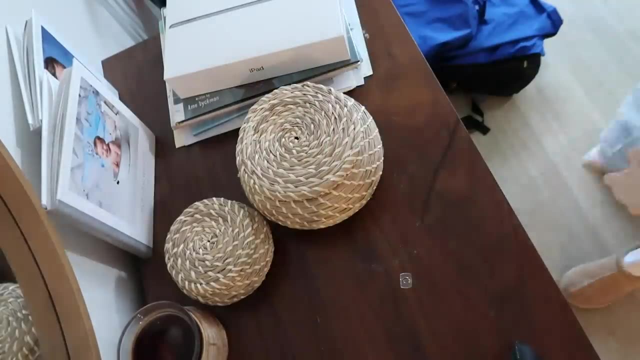 actually want to get rid of these bins all together. I think I'm not 100% sure yet, so for today I did just go through them and get rid of any junk that had kind of collected inside of them, but I'm pretty sure I'm also going to get rid of those bins pretty soon too. 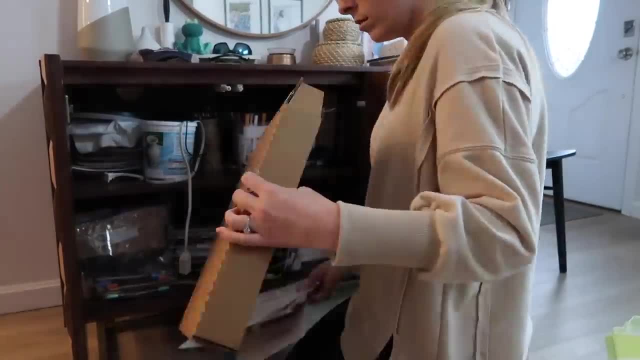 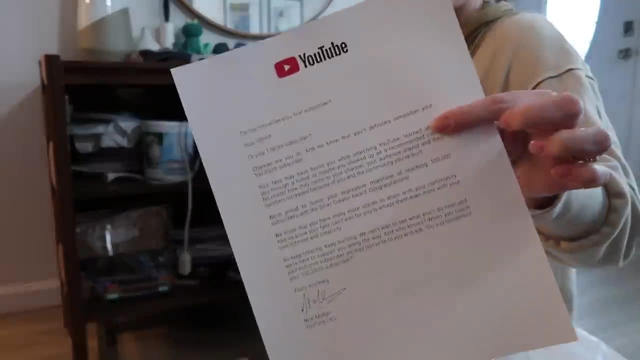 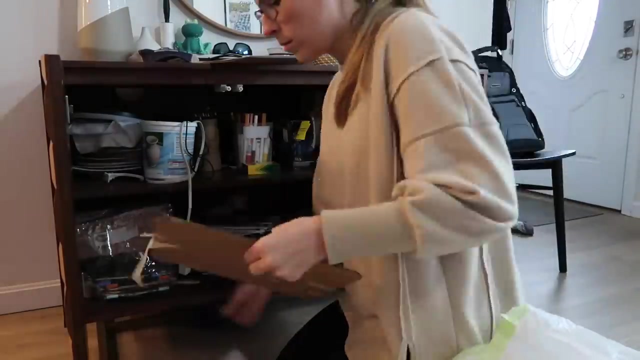 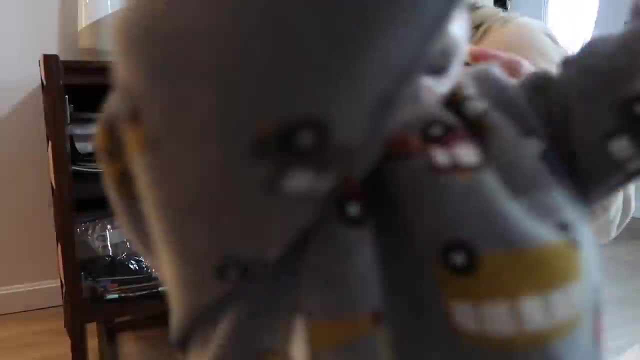 The inside of this cabinet I really wanted to store my kids art supplies. They have been doing tons of drawing and coloring and I've actually had most of the art supplies on an art cart in my oldest son's room. but now that the baby is really into coloring and drawing as well, you can 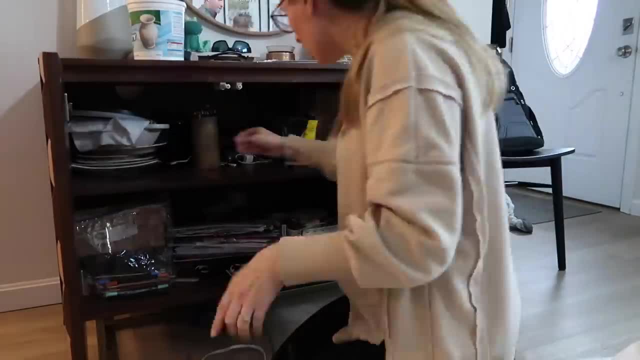 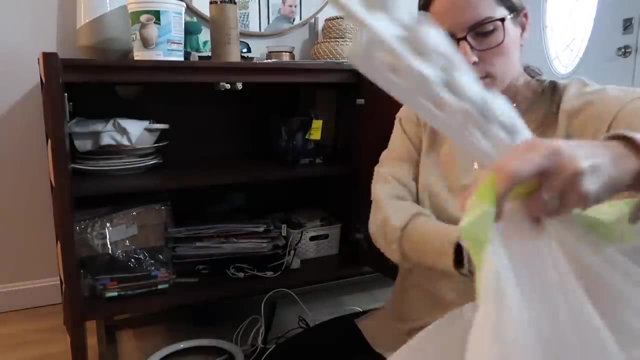 see, he just took out the markers. I wanted a place where I can put them back at the end of the day so I can clean off the table. So I'm getting rid of a ton of junk from inside of this cabinet. You'll see, I just keep throwing everything into this trash bag here so that I can make some space. 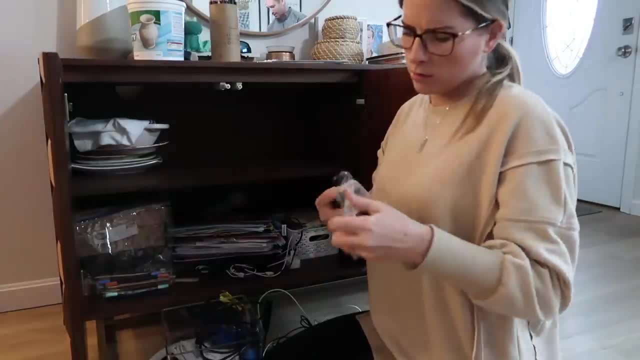 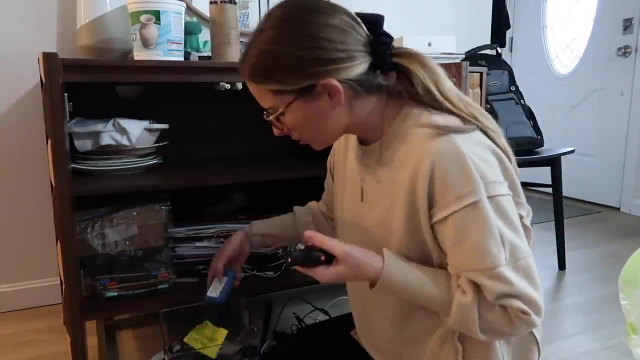 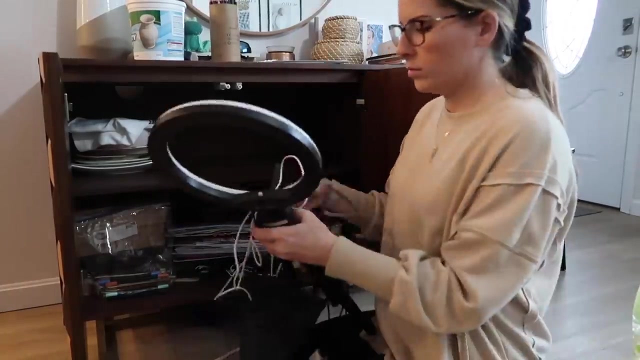 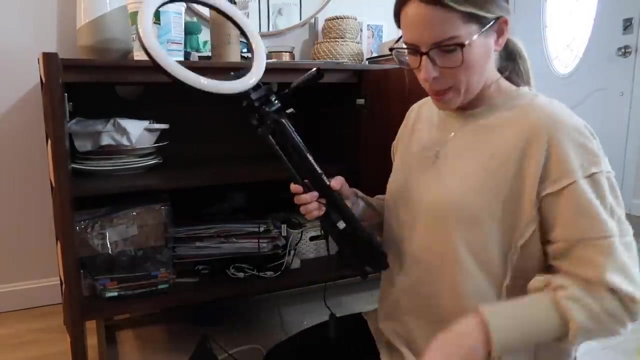 to store some of their art supplies and I'm so happy that I did this. There was so much clutter in here that we never use and we don't need and was just collecting dust and taking up useful space for other things. So this ring light was an impulse Amazon purchase that I made, thinking that I might be able to use. 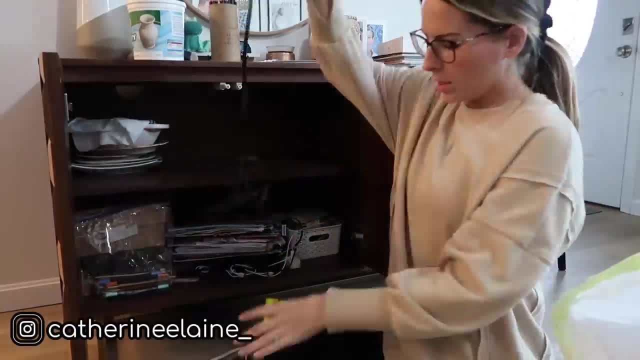 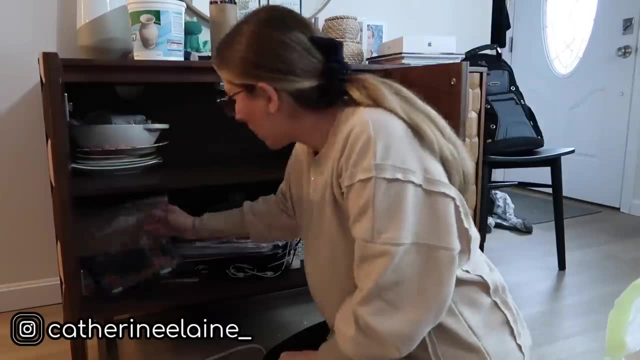 it to help illuminate some of my videos, but it truly is just not bright enough, It's not big enough and it just was not working, so I was never using it, So I decided to go ahead and get rid of that as well. but on the topic of Amazon impulse purchases, I really would like to cut back on. those as well in 2024.. Last year, my new year's resolution was actually to stop shopping on Amazon, but it is honestly so hard to do that. I feel like there's a lot on Amazon that they have that you can't find in stores, and it's also convenient to be able to have things delivered to your home in. 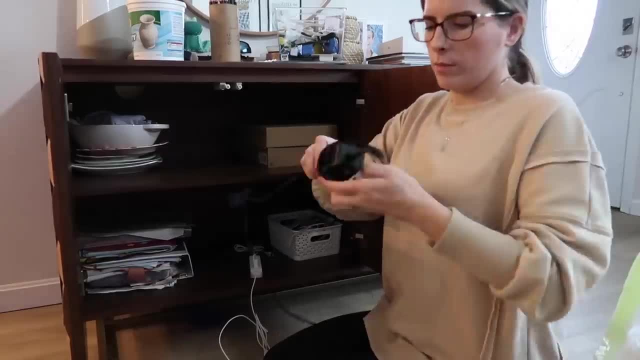 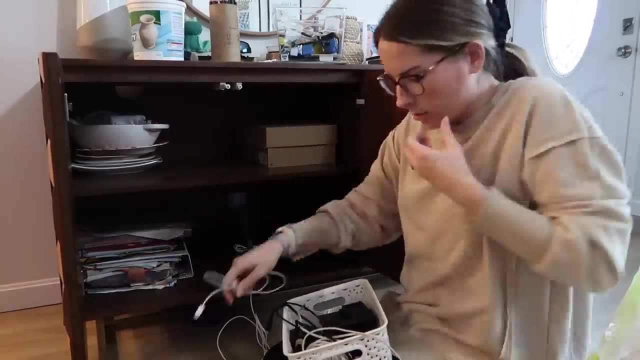 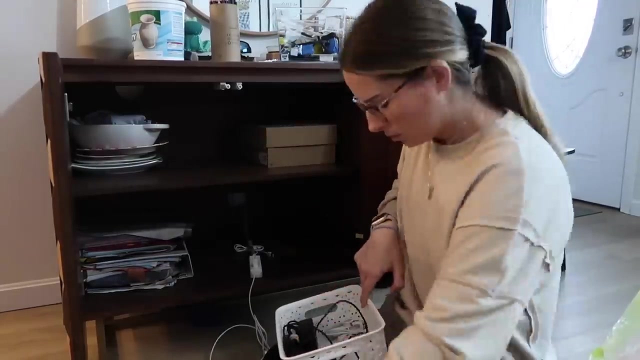 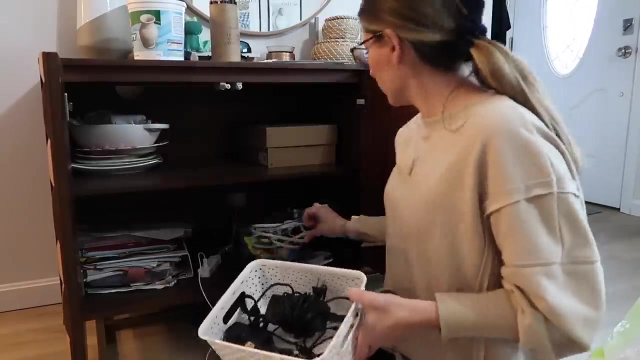 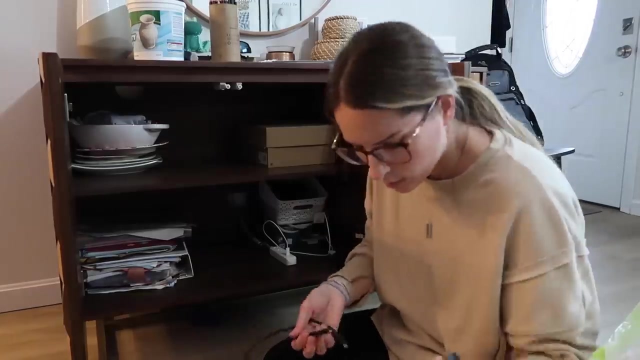 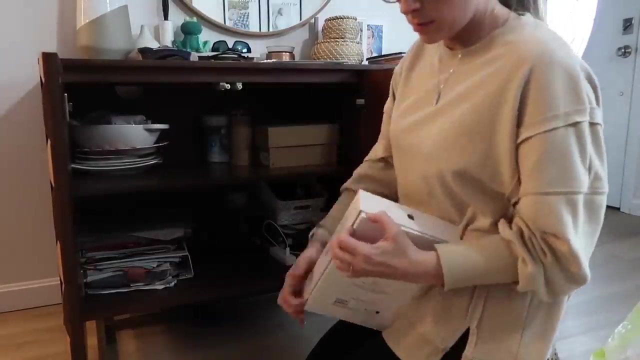 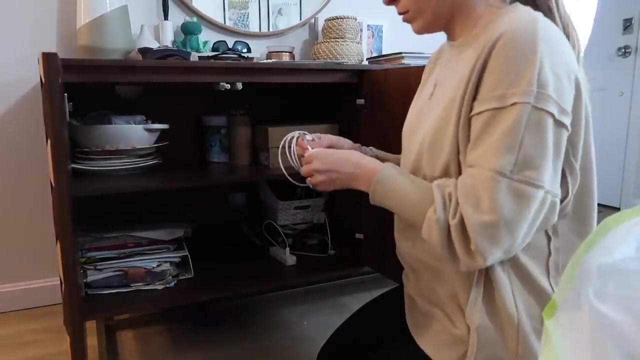 one day, instead of having to leave your house. So it has its perks, but I really want to be more mindful about exactly what I'm buying on there and whether or not I truly need it before I impulsively hit. add to cart. 🎶. Music Outro 🎶. 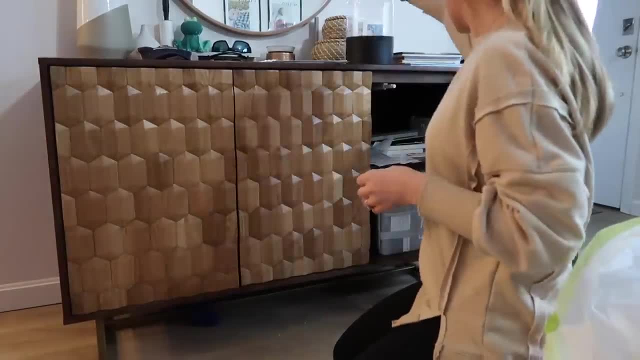 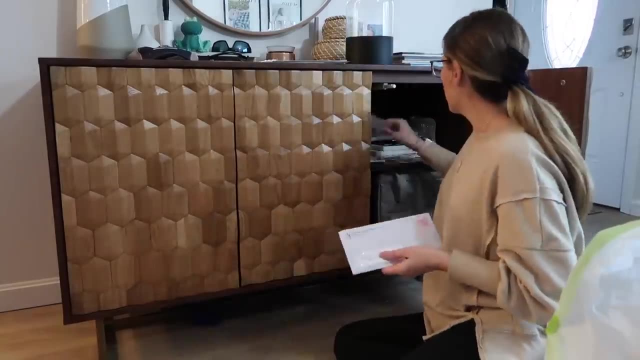 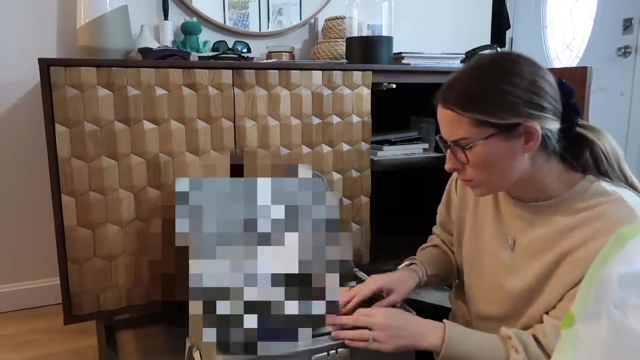 Now we're going through the other side of the cabinet. There was not much in there for me to get rid of, but for the sake of making sure that I'm covering all my bases, I wanted to go through this side as well and just clean it. 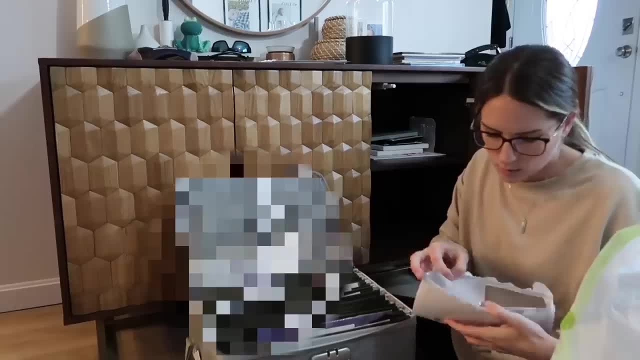 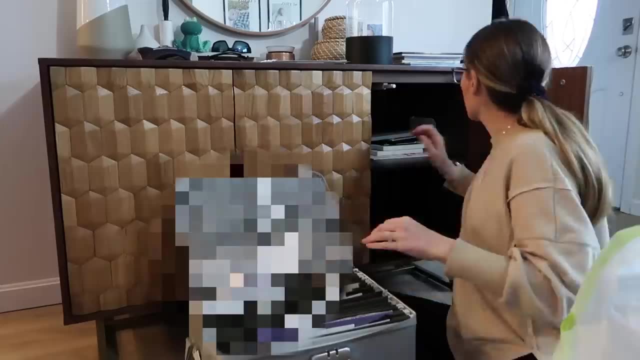 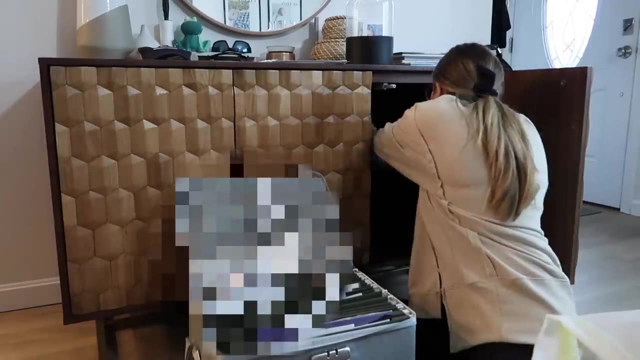 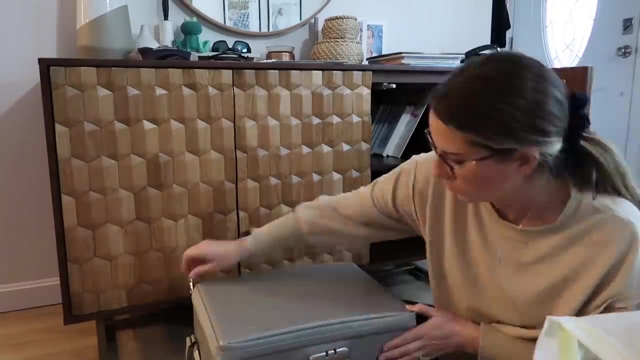 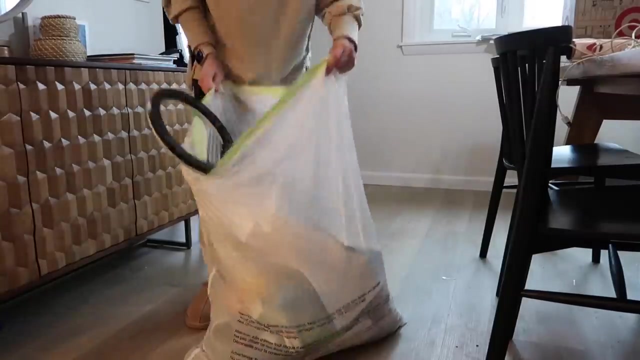 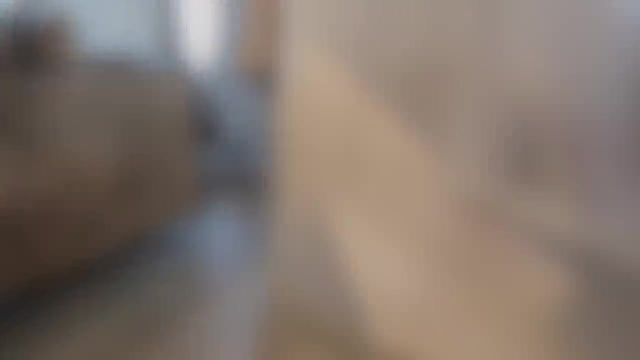 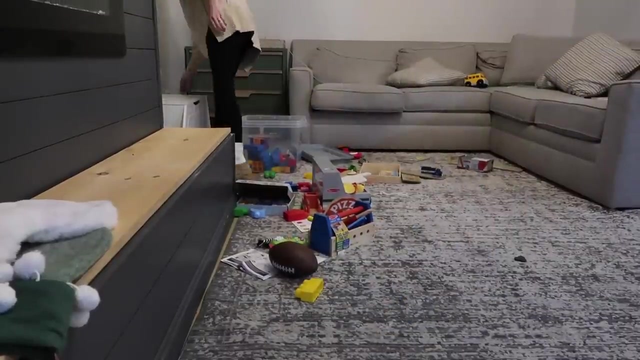 up And here is a big old bag of trash. All these things I was able to declutter out of our home and it felt so good. Now we're jumping ahead. to the end of the day, The kids were in bed and it was time for me to pick up for the night and I figured while. 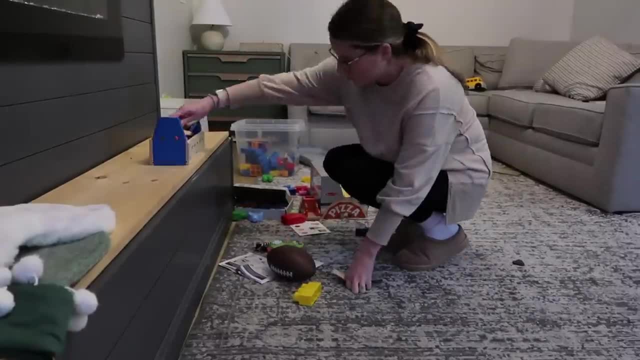 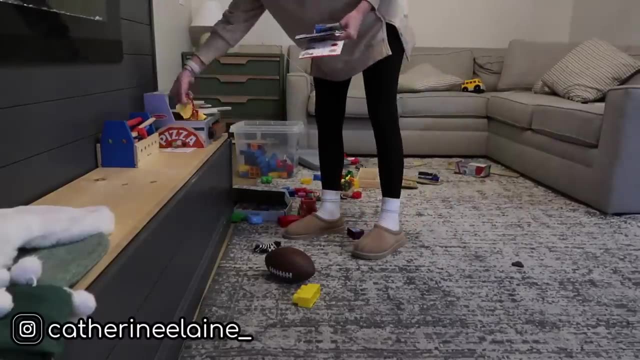 I was picking up, I would go through everything and see if there was anything that I needed to get rid of, And there wasn't a ton, but I had already decluttered an entire trash bags full of things, so I definitely felt like I accomplished. 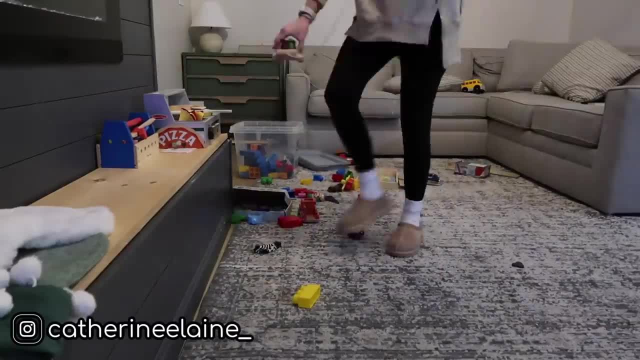 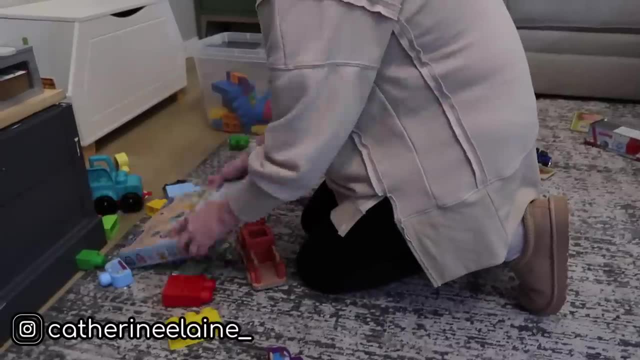 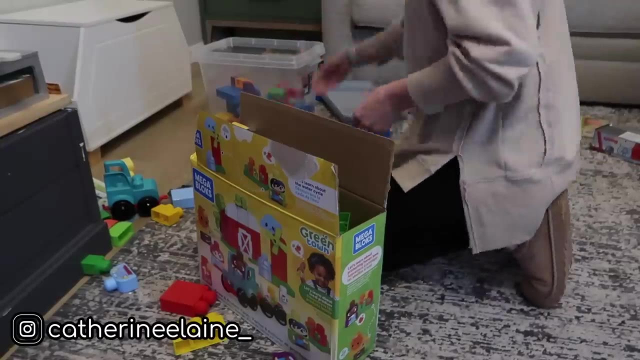 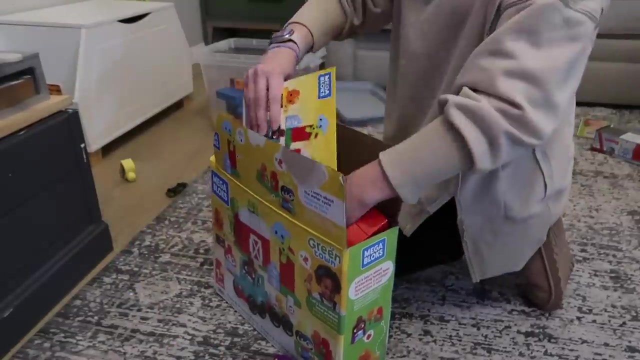 a lot of decluttering in this day and I was super proud of myself. I already did a big declutter of toys before Christmas. so if you need any toy decluttering motivation going into this year after we've just finished the holidays, I will have that. 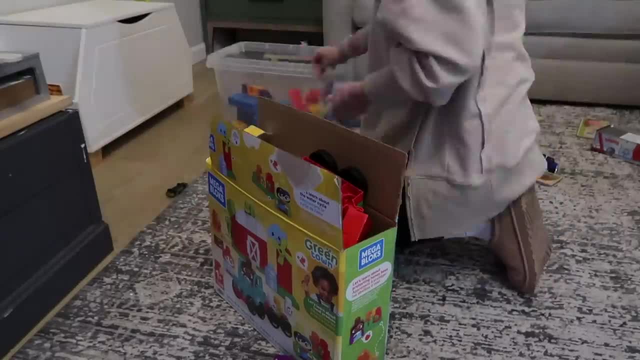 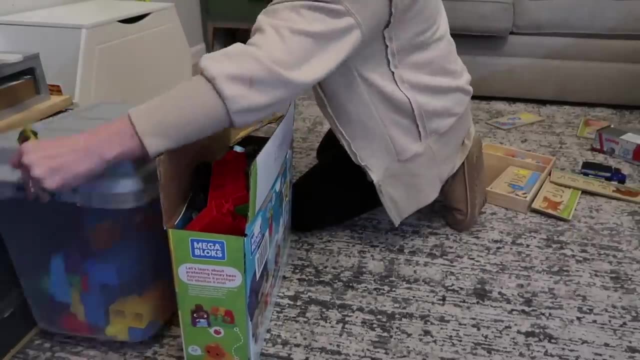 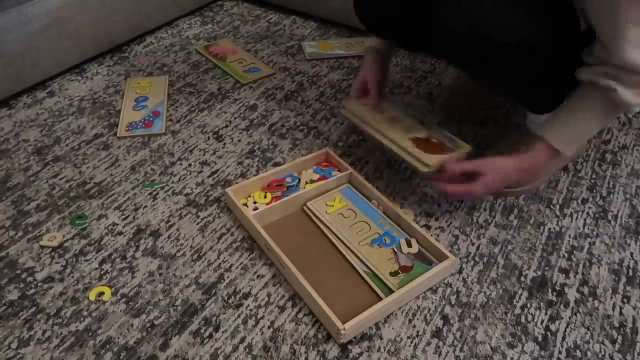 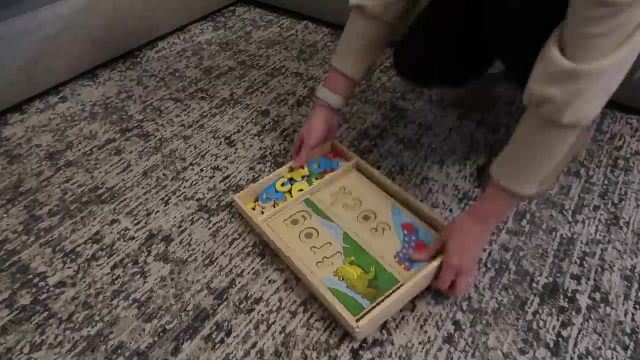 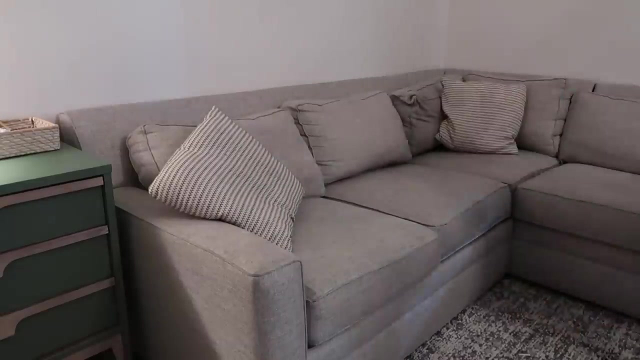 linked in the cards right here, So hopefully that helps you. If you have any questions, let me know in the comments below. I know you are struggling right now with all the extra inventory that came in over the holidays. As of the day that I'm doing the voiceovers for this video, I have taken down all of the 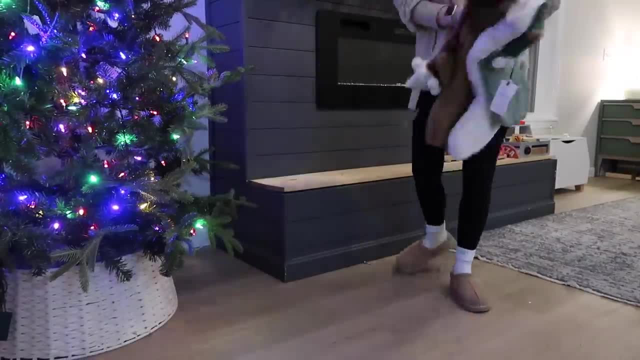 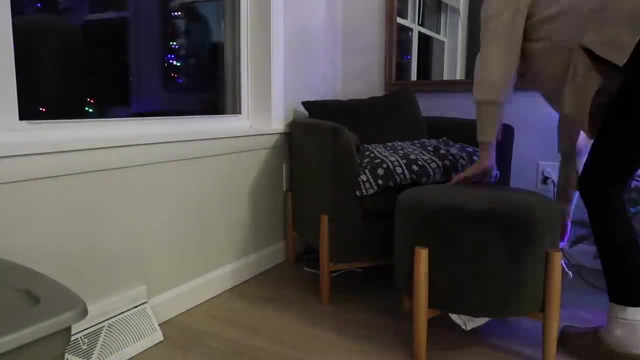 Christmas decor, but I already kind of miss it. While it is definitely clutter around the home I love all like the lights and just how cozy it feels. So I don't know. this year I was really enjoying our Christmas decor and keeping it up a little. 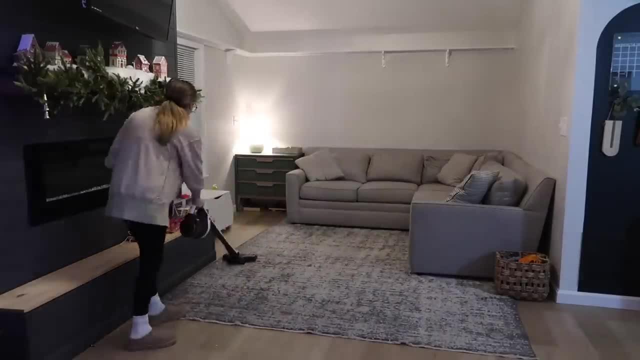 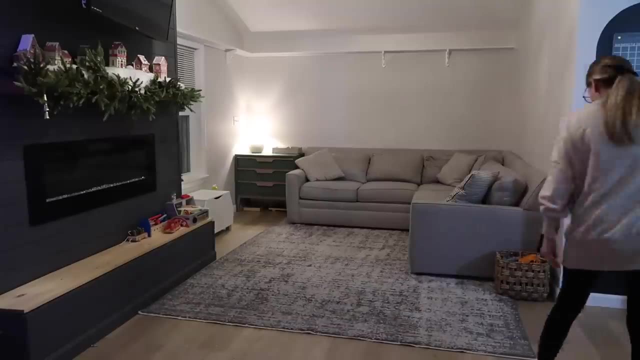 bit longer and just how cozy it felt, and I think part of it probably had to do with our beautiful fireplace that we built in 2023, but it is all down now and I feel like when I'm cleaning up at night, it's just not as cute anymore. 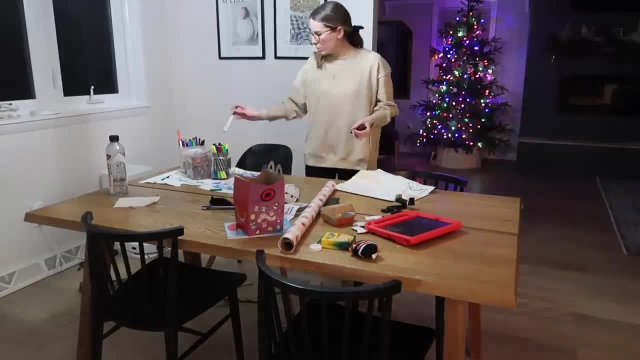 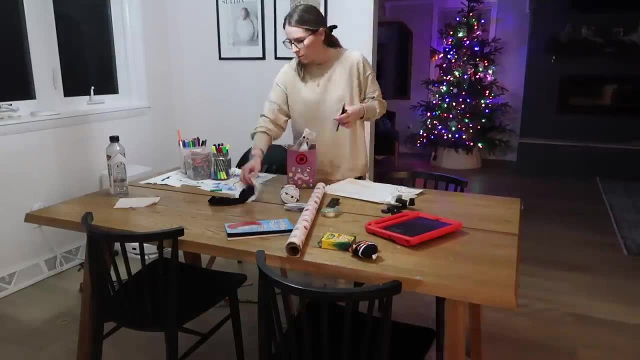 So, like I was saying earlier, my kids are very into drawing right now, So my dining room table pretty much always looks like this because they're constantly coloring, So I wanted to clear the table off. there was definitely some things on here that weren't. 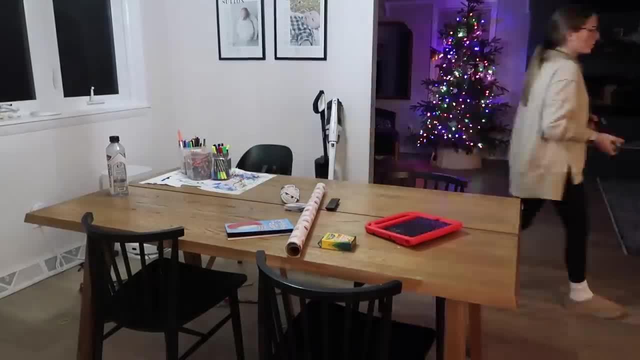 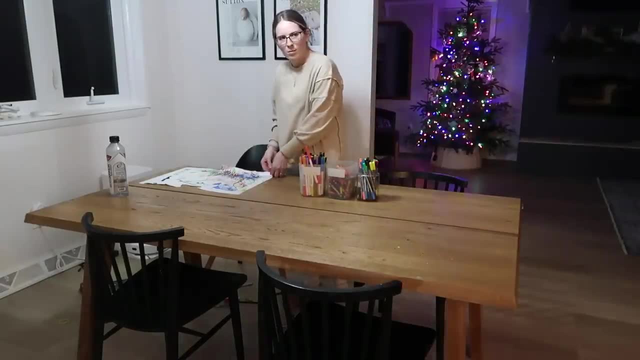 art supplies wanted to get those back where they belong. Like I said, this was a couple days after Christmas, so our house was still kind of in shambles after the holidays, but I was really excited to be able to put back all. 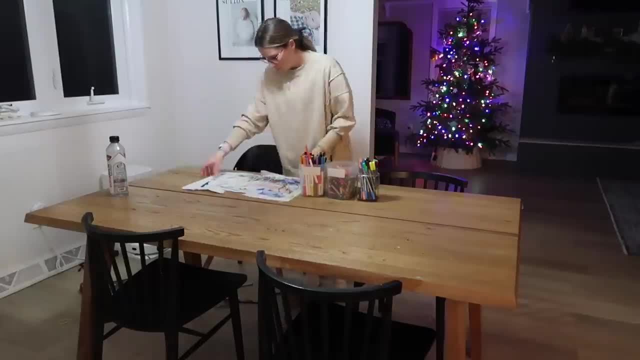 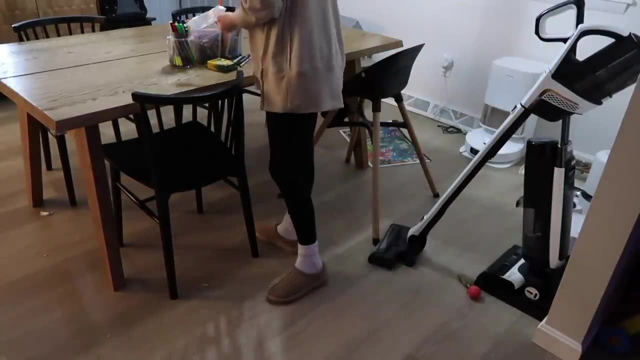 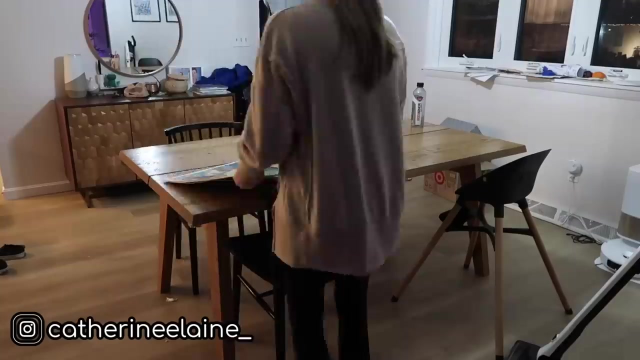 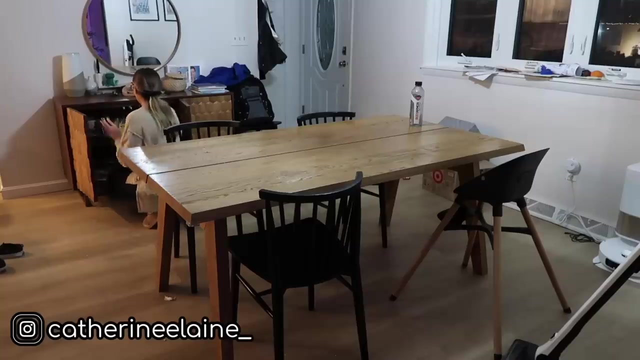 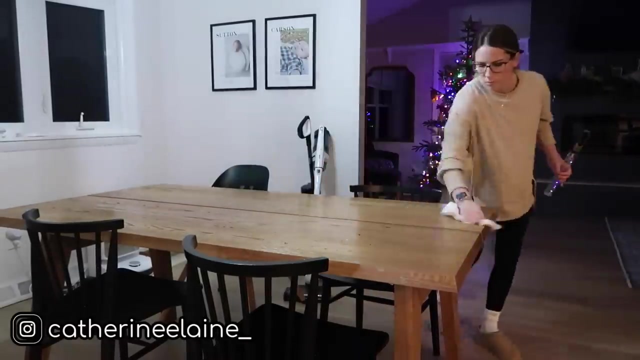 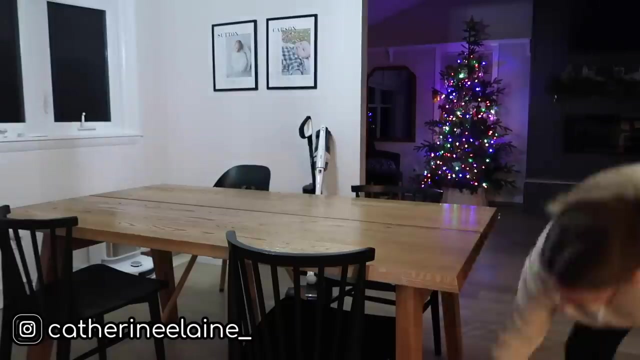 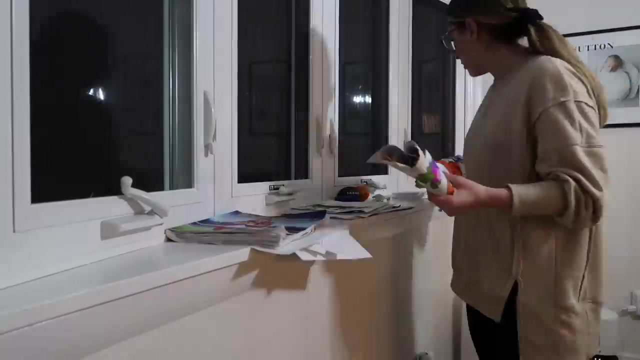 of the art supplies into that cabinet and have somewhere to put them at the end of the day when I'm cleaning off the table. I wanted to go through this pile that had accumulated on our windowsill. I don't know what it is about this windowsill, but we love to put things there. 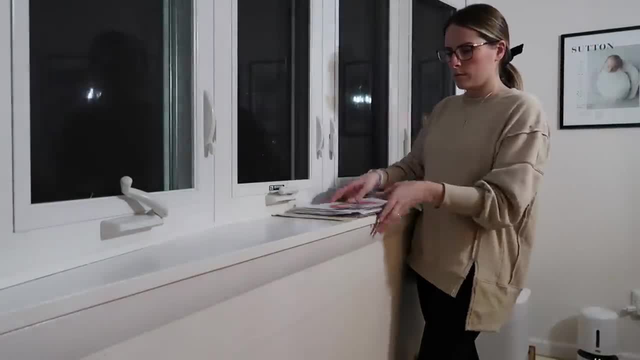 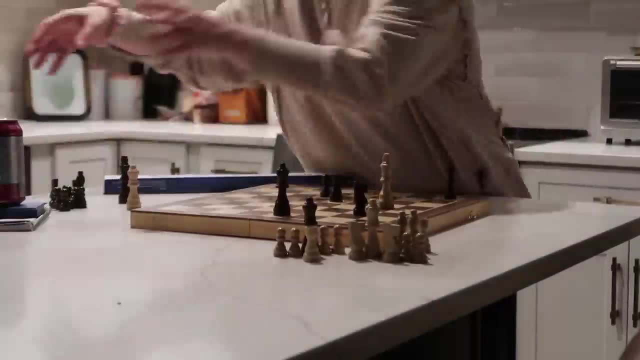 So I was going through the pile seeing if there was anything that I could get rid of. Some of this was my son's artwork that I didn't want the baby to be able to grab, So I just kind of stuck it back up there, but that's obviously not a permanent home. 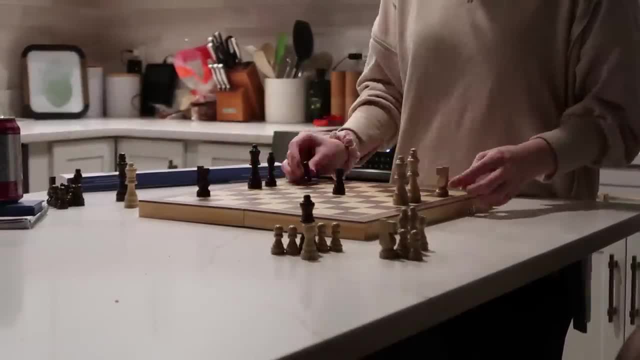 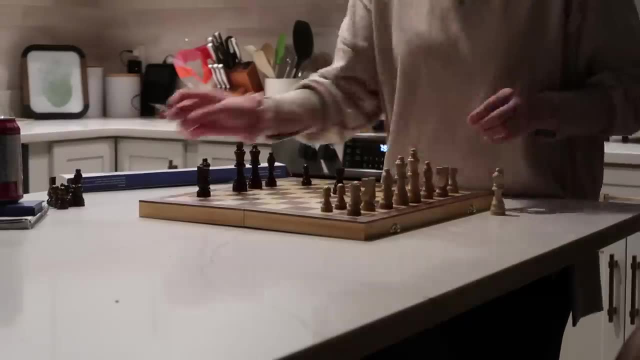 This chessboard was a gift for Carson, our six year old, for Christmas, and we have been playing so much chess and it's been so much fun and i didn't want to fully put this away, but i wanted to at least set it up so it's ready to go for the next time that someone decides to play it. 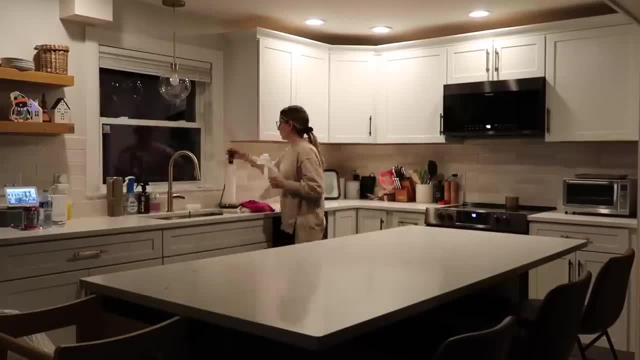 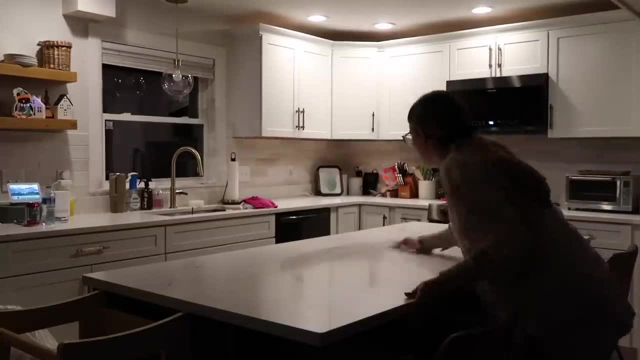 now i am cleaning off magnets off of the fridge. we have had those magnets forever and they've been a hit with both of my kids. i'm also going to clean off the countertops and then we'll get to doing some vacuuming. and speaking of vacuums, that is something i also don't plan to purchase. 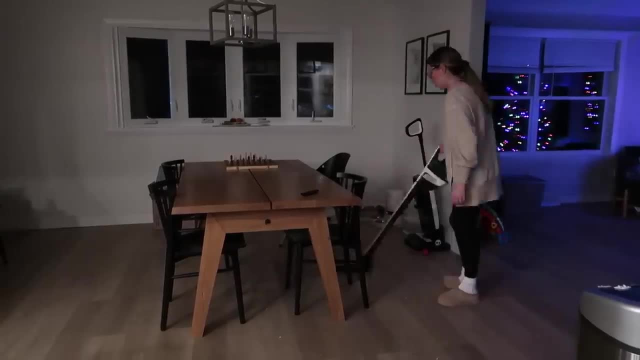 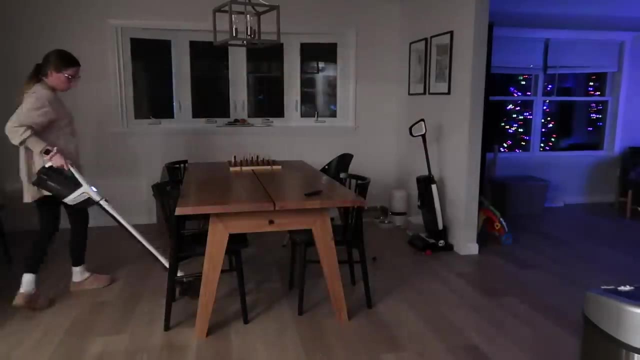 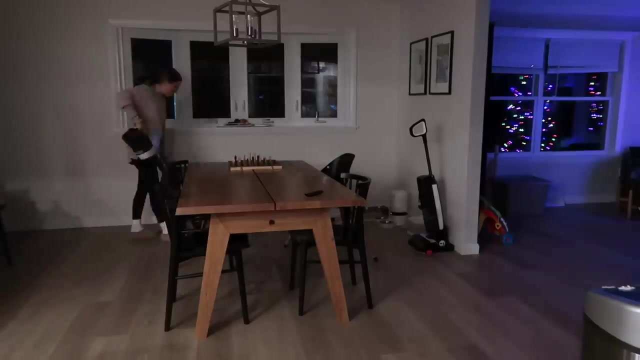 in 2024.. sometimes i do get sent vacuums and different cleaning products to feature them in my videos, and that is one thing, because that's just a part of my job. but i personally don't plan to purchase any more big cleaning tools in 2024, because we just don't need them. 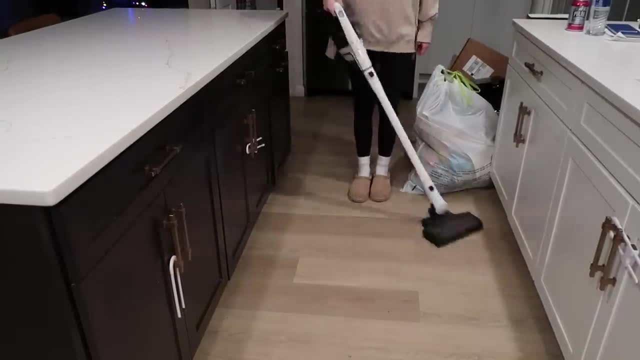 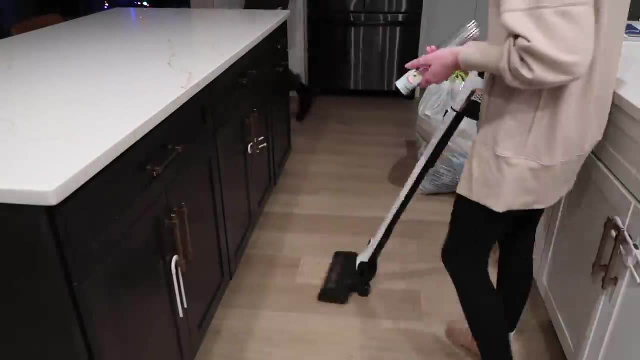 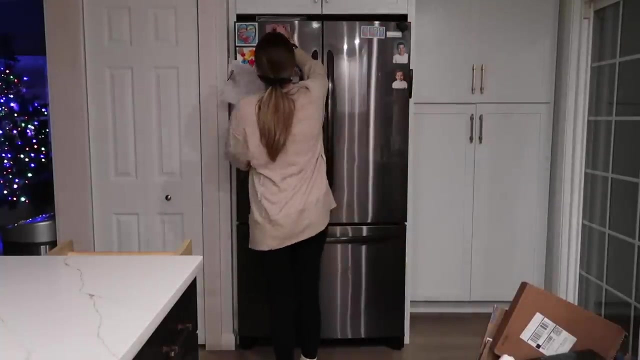 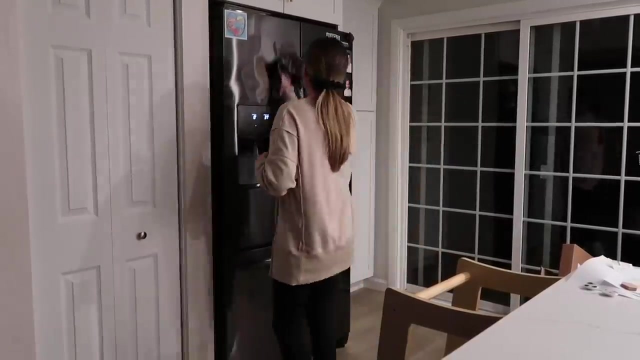 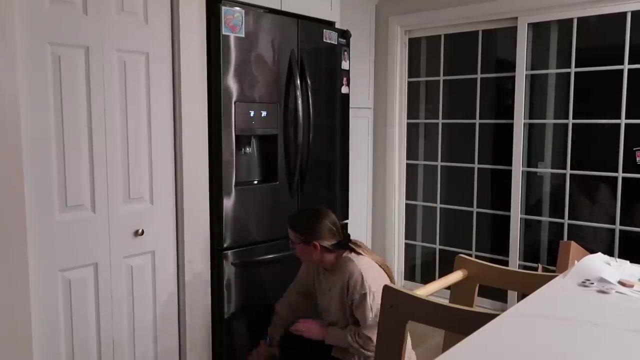 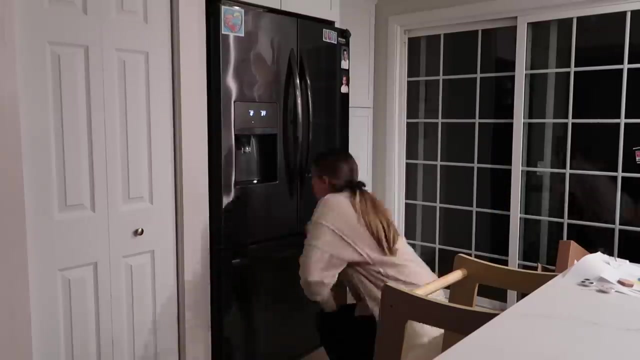 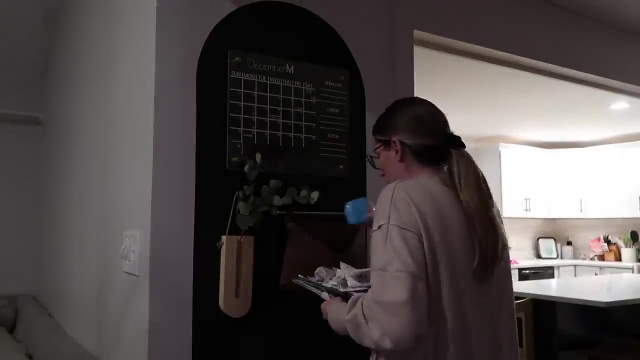 you would never be able to tell on camera. but our fridge was disgusting. it was covered in sticky little baby fingerprints. so before i felt good about stopping for the night, i wanted to clean the fridge off. so i stepped out of the Orient and carrying my Congratulations, the last thing that i wanted to do was declutter our little envelope that we use here on our